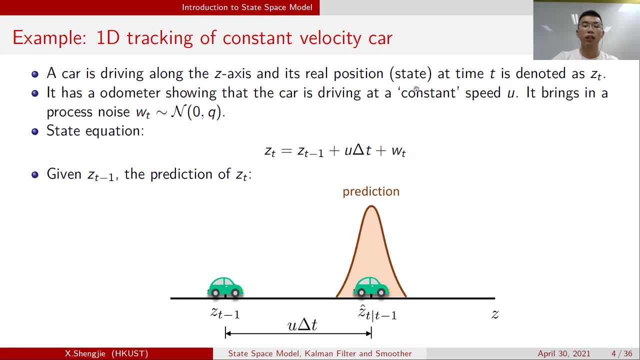 When you imagine when you're in a stock, then whether the stock is bull market or not, it itself is a hidden state. Hidden state means some information that you don't know, you don't really figure out or observe And consider. a car has an odometer. 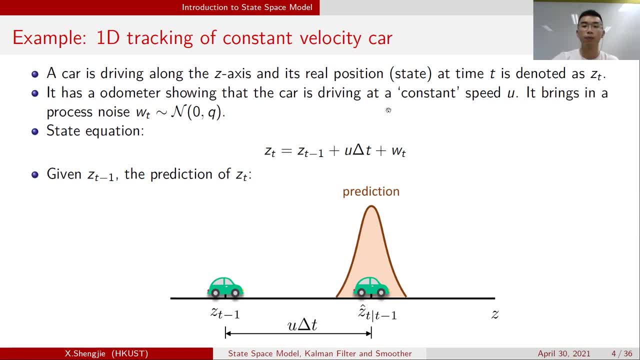 showing that the car is driving at a constant speed. u And because this odometer, which is the measures of the velocity of the car, it's like a panel And it will bring in a process noise which denoted as wt, And then the hidden state. 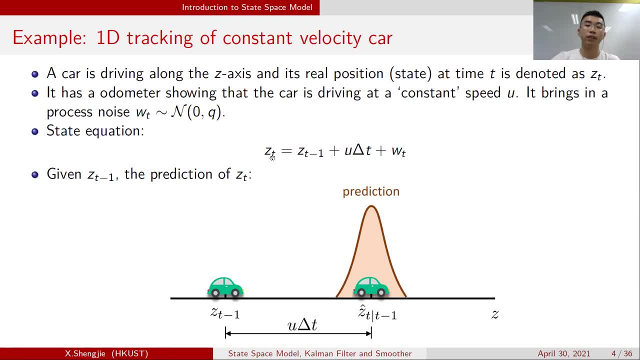 we have this equation: The position of the car at t time. t is the position of at t minus one, plus the velocity multiplied by the time period, And also add up a Gaussian noise. So using this equation, we can make a prediction at t minus one. 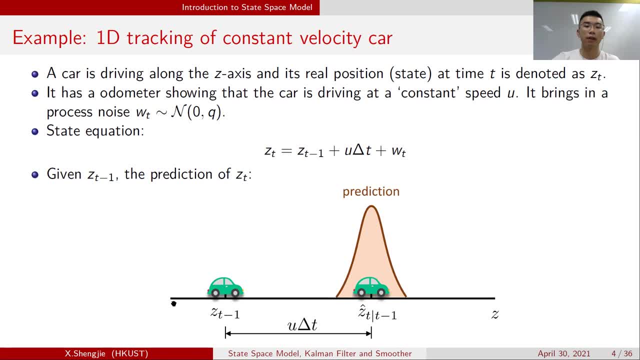 on the location at t, For example. now the car is here, we can make a predictions on of our car at t, And it will look like a bell because it follow a Gaussian distribution. And so this is is describing how the 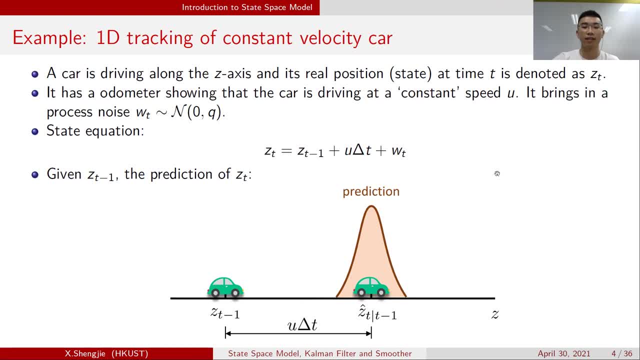 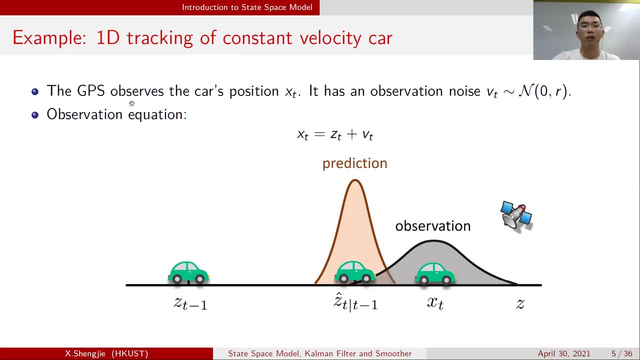 the car is is driving along an axis And then simultaneously we have a GPS, which is a sensor. It will observe the car's position And its observation is denoted as x. So you should make a distinction between x and z. 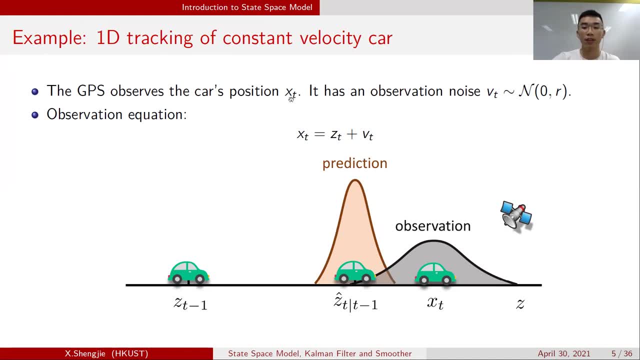 Z is real position, but x is the observation. These observations also has a noise. For example, there are five meters noise, and so on. So the observation equation will be look like this one, which means our observation is in fact the. 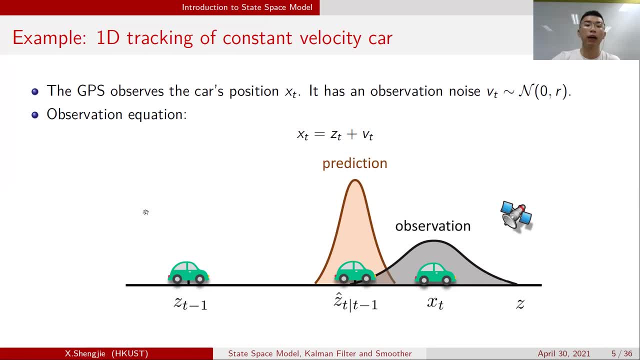 the real position plus a Gaussian noise. So in this graph you can see that this one is the prediction and this one is the observation. They may not be the same And the problem comes up: How to find out the real position of the car. 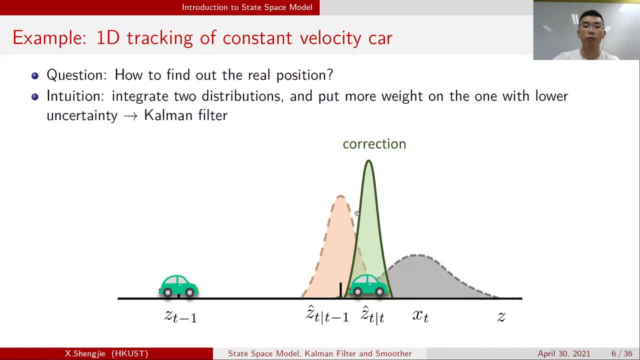 We don't know. We don't know the real, exactly, the real position, But we have the prediction and the observation. In this case, we can simply integrate them together. Integrate these two distribution together and put more weight on the one with lower uncertainty. 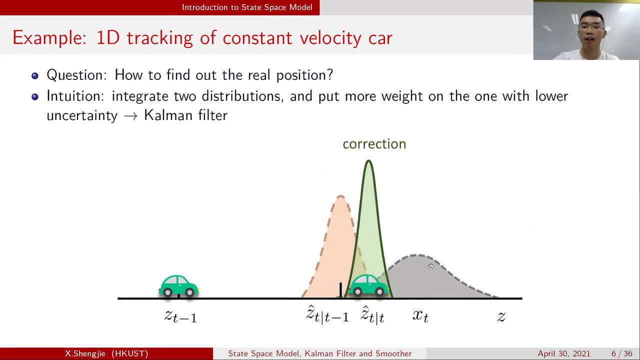 You see, this one, the Gaussian, has a lower uncertainty. This one will have a higher uncertainty. So we would trust more in the prediction instead of the observation. So, in fact, this is the ideas of common filter, and we will talk about it later. 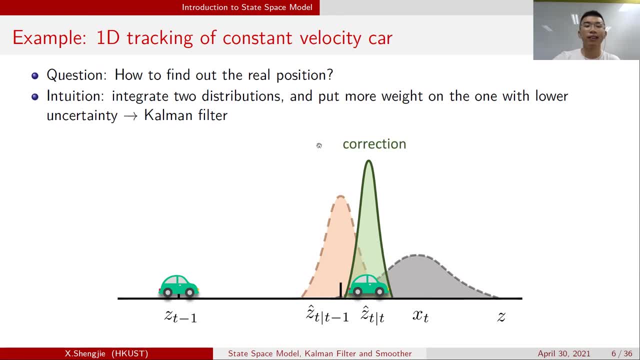 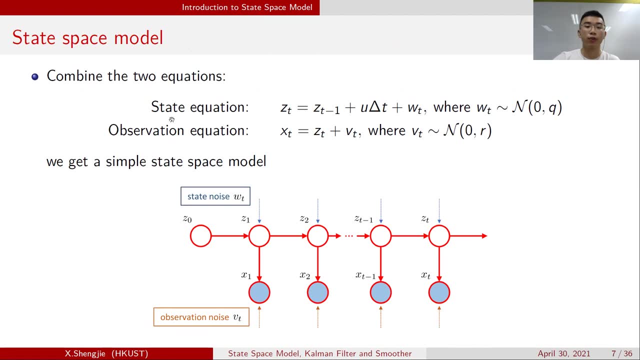 So these pictures should be in mind. Yeah, let's continue. In the previous example, we write up two equation, which is called state equation and the observation equation, And we put it together. As you can see, it's a really elegant form. 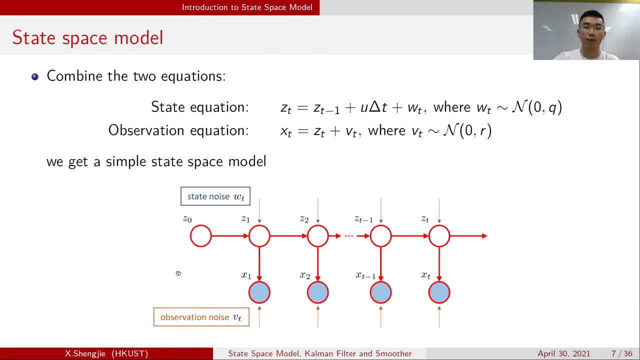 And we can also draw it out like this graph. As you can see, the state which is the hidden location or the real location of the car is in fact follows a chain. Each node is only dependent on this previous node. 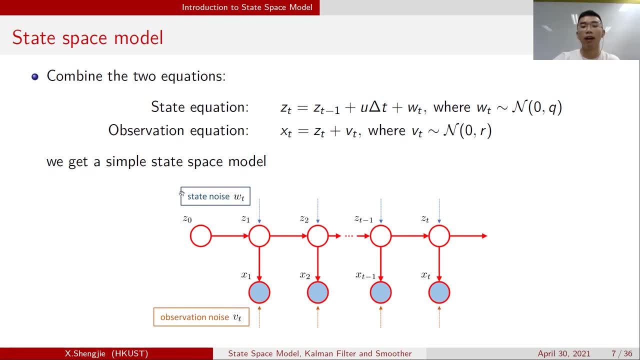 but not on the nodes, that is before. So it is in fact follow a marker of property And each observations. we only depends on this relevant state, relevant hidden states. So this is how we illustrate this equation And 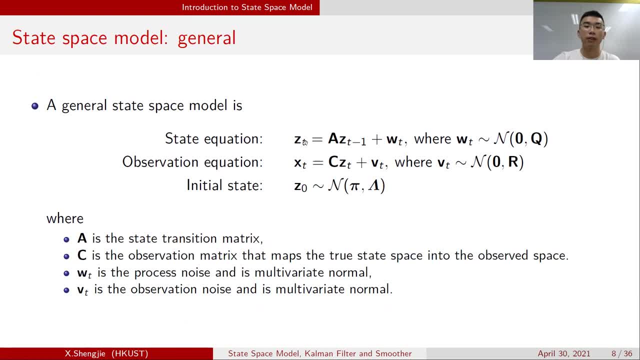 more generally, a state-based model will consist a transition matrix or an observation matrix, which try to map the state base into the observed space. The two space can be different. What you observe can be something like acceleration or latitude or something like that. 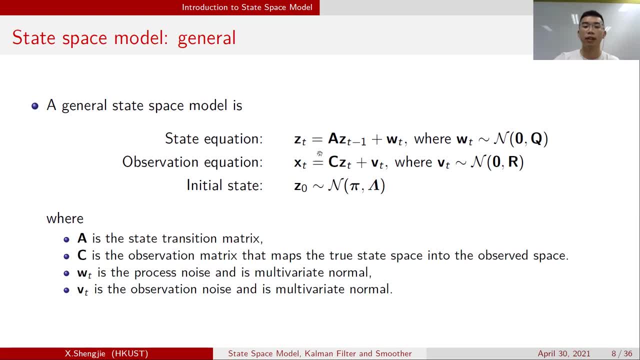 But they don't exactly to be the position of the car. So there is a linear transformation here And this state can be. there are multiple, can be multiple space, So multiple states, So it can be a vector. 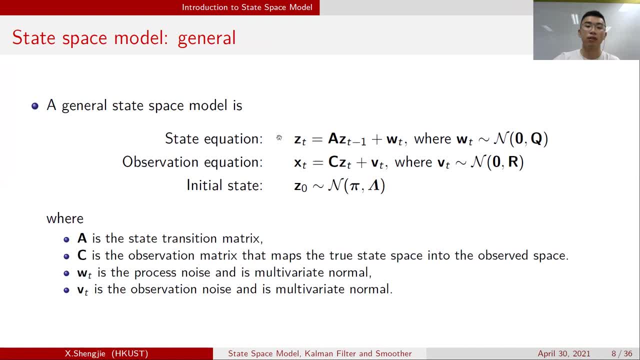 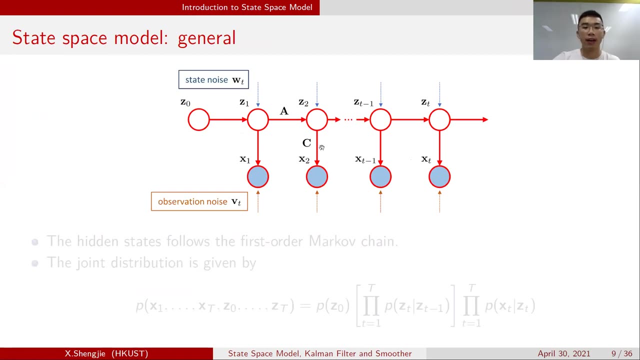 The observation can also be a vector, meaning that there are multiple sensors recording the position at the same time, And so this is a more general waveform, nothing special compared with a previous one, And this graph will look like also almost the same. 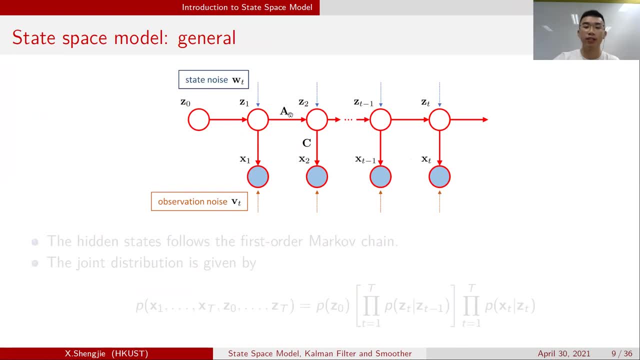 but with a matrix here. The A here means the state transition has a linear combination relationship And the C here also has a, has a relationship, projection relationship. And from this graph we want to highlight that the hidden state follows a marker. 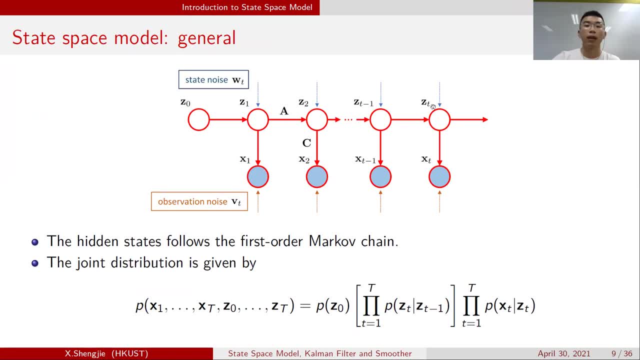 a lower marker property, And, and which? what was the benefit? The benefit is that when we want to write down the joint distribution of the state and the observation, we can simply write down like this: The the distributions of the initial state. 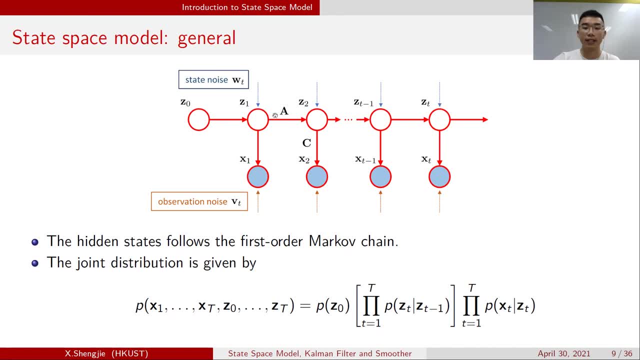 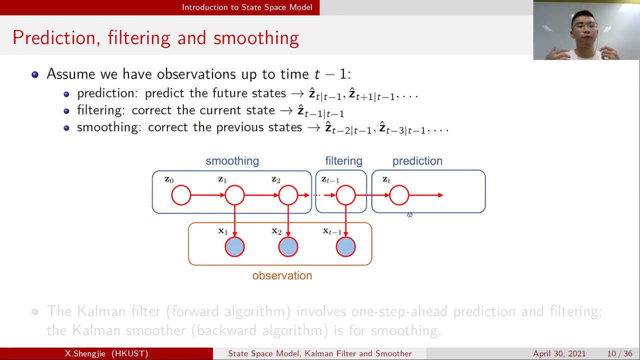 multiplied by the cross products of how the state transit And also multiplied by how the observations occurs. So this is a really elegant form of the probability. And so, before we go to the common common filter and common smoother, 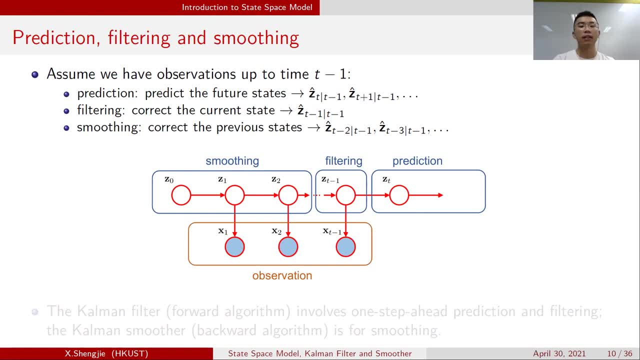 I want to clarify three concepts here. The first one is called prediction. Assumes that we have already observed T minus one observations And then when we want to predict the state at T, it is it is called prediction Or predict the state that. 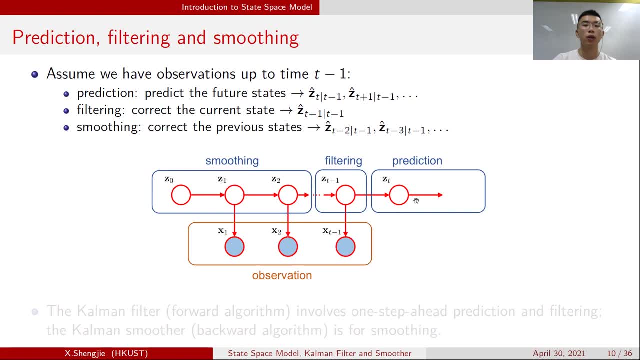 in the future like T plus one, T plus two. this is called prediction And filtering means. after we have observed these T minus one, we want to. we try to update our current states, our state T minus one. 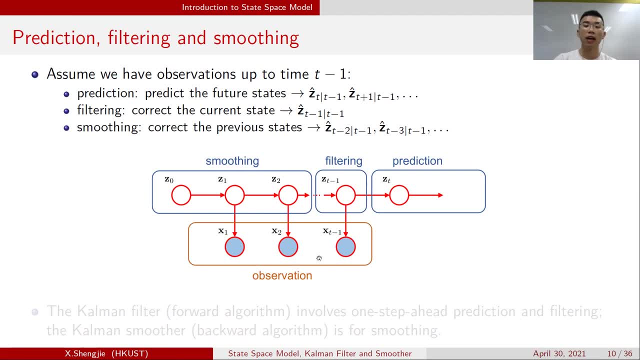 Because in previously we have predicted one, but because after we have observed, observed the, the new observation, we can try to correct its, its prediction. This is called filtering, And smoothing means we try to. 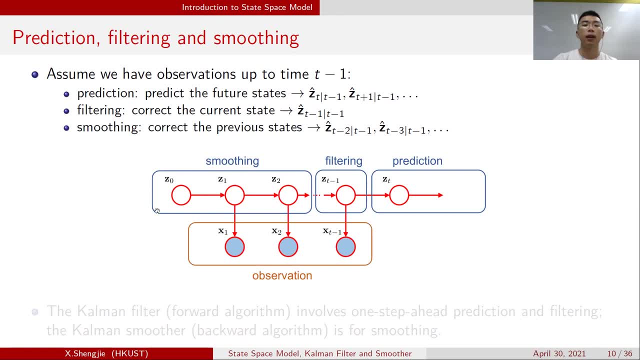 update previous estimation of the state. So these are three concepts, So filtering and prediction. when they combine them together it will brings in the what we call a forward algorithm, a forward flow. Forward means each time we will. 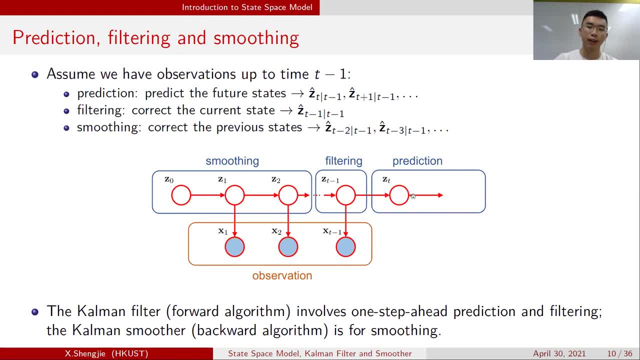 we first, we predict. for example, we first predict and then, after we observe XT, we try to filter it, And this is called forward. We are always looking forward And look, and so this is the concept. 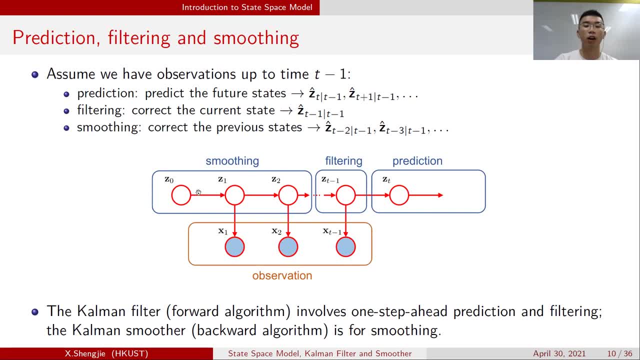 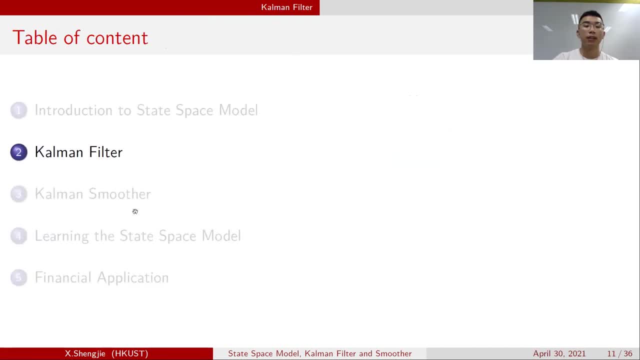 of common filter And the smoothing is achieved by using common smoother. It's it's trying to do the backward flow. And so let's get in the details of common filter. Common filter is, common filter is is first: 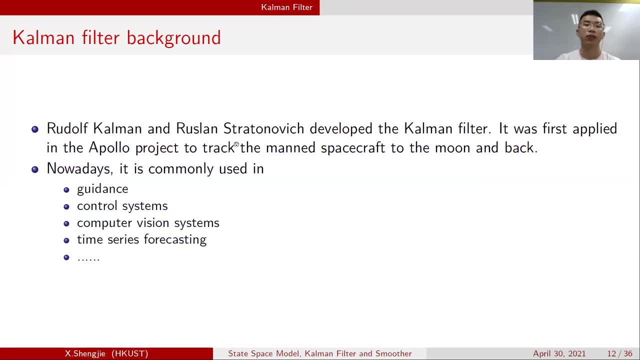 designed by the, the guy Carmen and also a Russian business, And it was first applied in the Apollo project And they are used to track the many spacecraft And nowadays it's widely used in many areas. 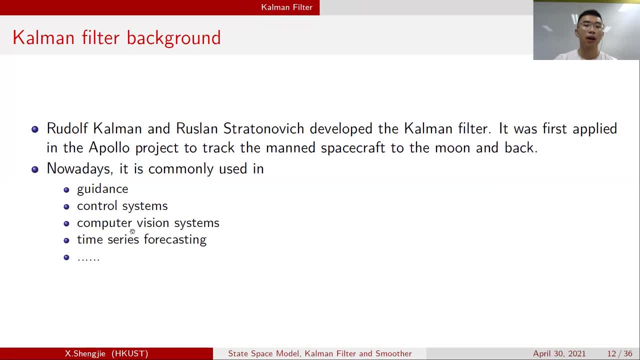 like the control system or the computer version system And I think for our students, more importantly, it is used. it's quite useful in the time series forecasting And with this Davis model we can forecast the price. 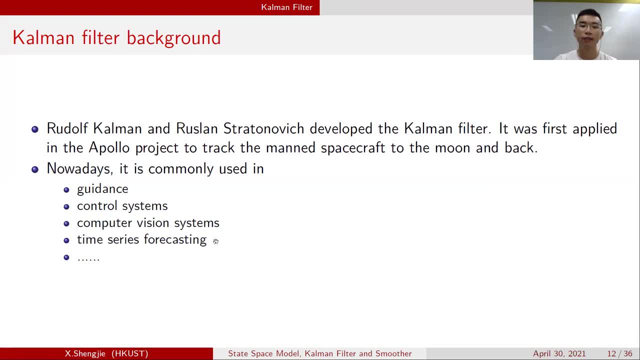 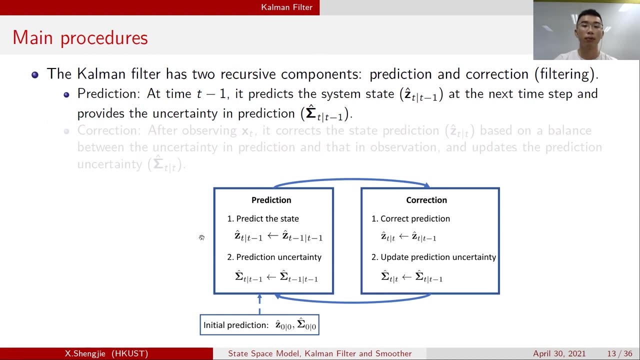 we can forecast the volatility, we can forecast the trading volume, as we can. we will see later, in later chapter. And so this is the backgrounds of common filter, And common filter is simply composed of two components. First one is called prediction. 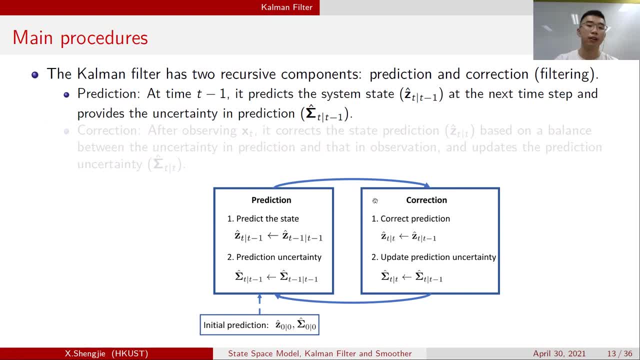 and the second one is correction. as we have shown shown previously, Prediction means, at time, t minus one. we will try to predict the states at t. So this is the denotions of, of of this estimation. 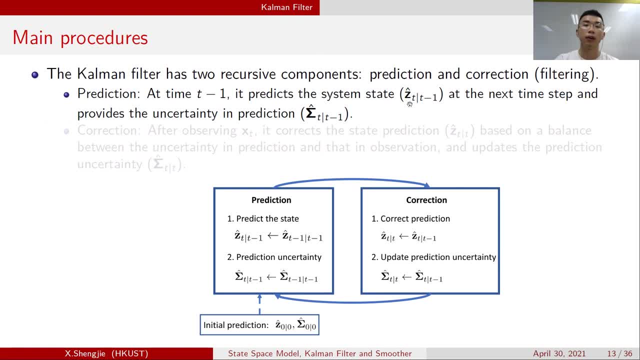 T they. t means our estimations of of the state at t conditions on t minus one observations, And we will also provide the uncertainty in the prediction which is the balance of the of a Gaussian function. 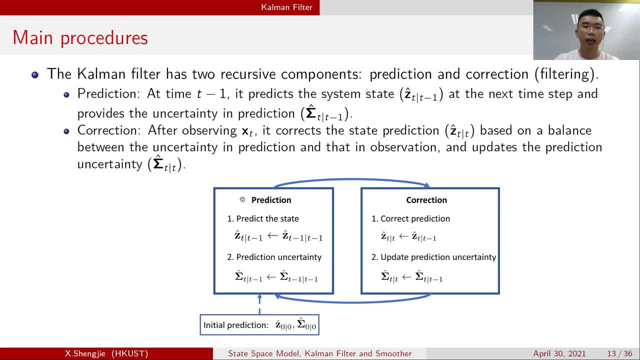 And the next set is called pre correction. Correction means after we have observed X, t, the, the observations at time t, we will correct our state. we will correct this because we have estimated this one And. 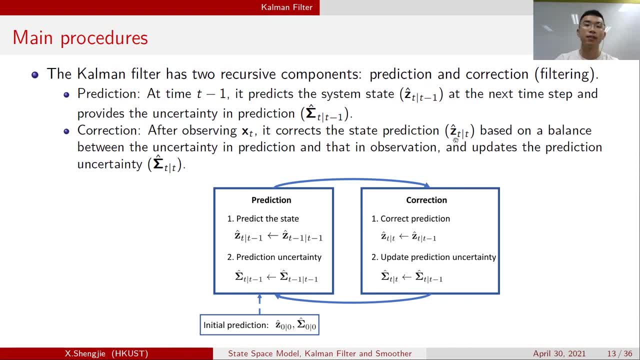 we want to correct it And you would have a denotion like this, which means our estimate, our corrected state at t at time, t condition on all t observations, And we will also try to update. 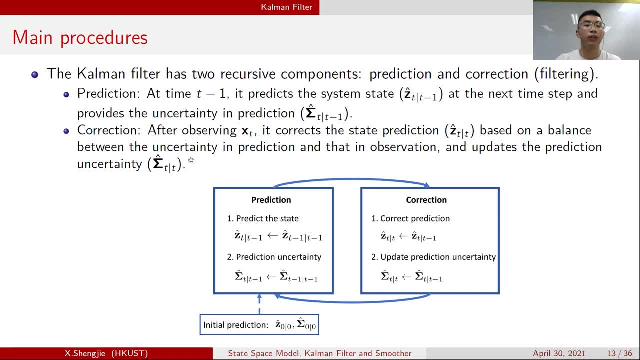 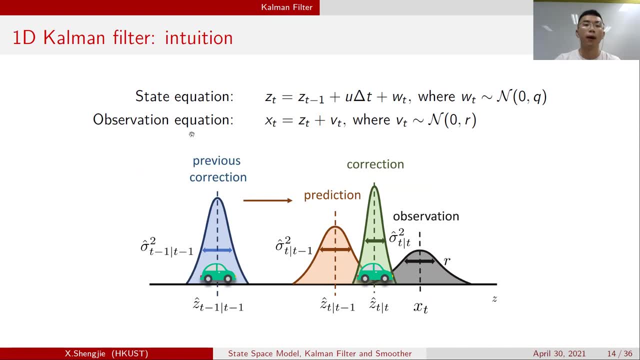 our prediction uncertainty denoted as this one, And let let's see how it works. in our previous example, Our previous example, the state-based model is is placed here And we have a previous correction: assume at t minus one. 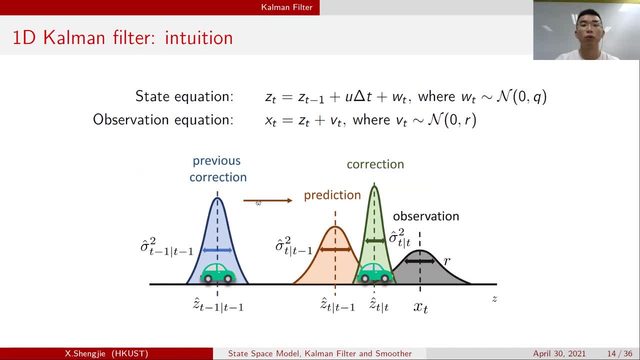 we have a previous correction. The first step of common filter is doing prediction. It will predict then what the, what the car's precision look like in in the next time step at time t. So this will be a bell. 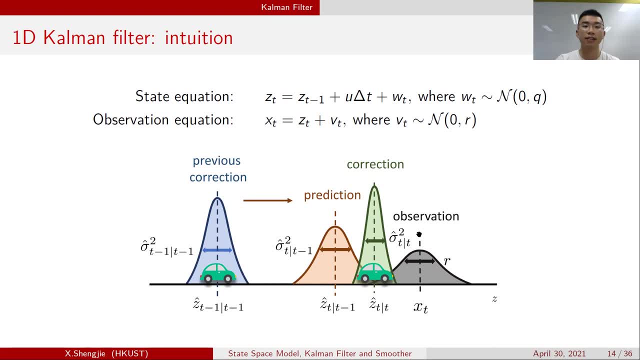 And then we observe at time t, we observe from, from the sensors, So we will have another, another bell. So the problem, as you can see, this one, the, is variance or is uncertainty. 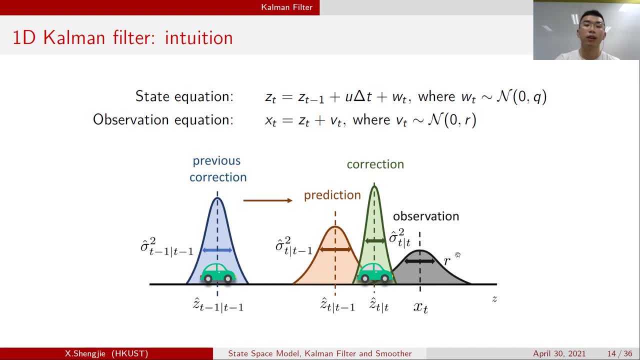 is defined as this And the observation we have, the observation noise, is defined as r. So the problem is that how we do the correction to find out the find out the, the real position. So 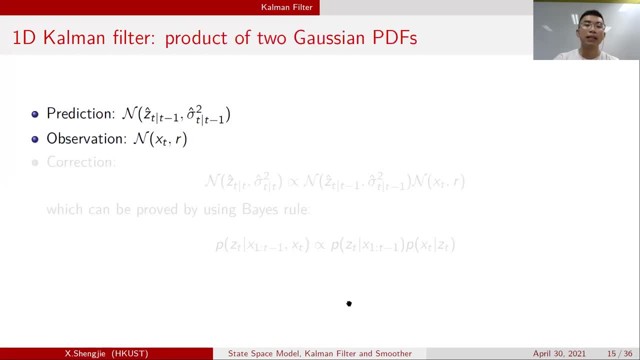 in termsly with these two Gaussian we have, we have already have. we will do. the correction is by simply multiply these two Gaussian PDF or Gaussian function together. You might, you might think okay. 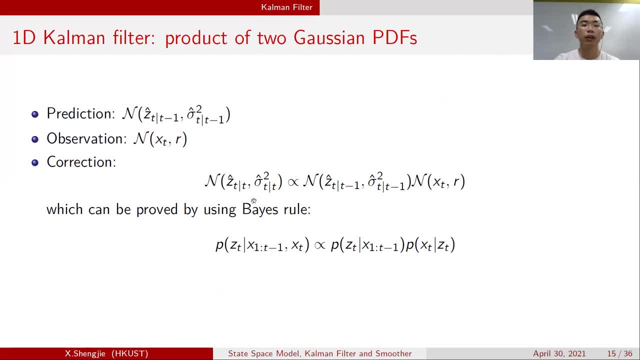 it is. it's so heuristic, but in fact this is, this is, this is, but in fact there is a proof, by using Bayes' rule, to prove that this one is valid. So 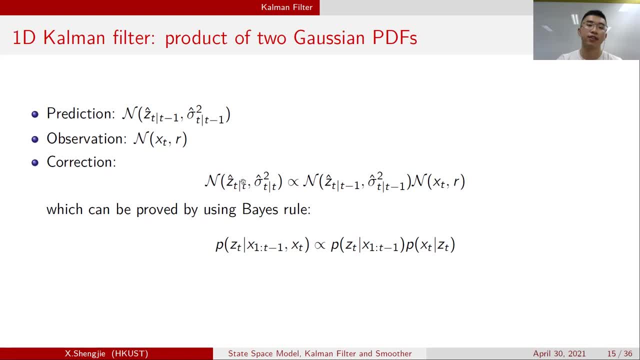 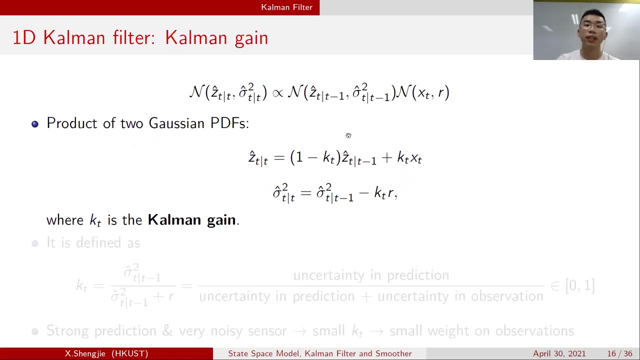 try to remember that the correction is in fact the corrected Gaussian is erected is in fact the, the modification or the products of of the prediction and the observation. And so let's go into details. 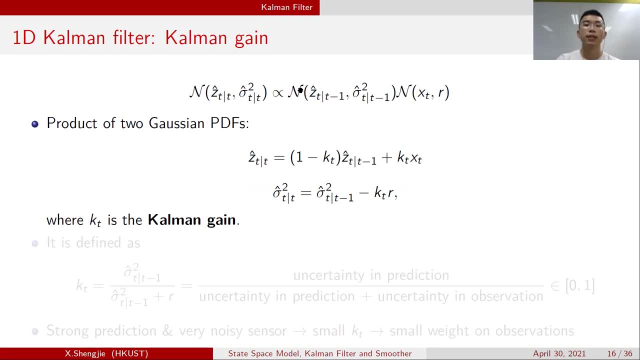 of these multiplication. As you can see, the expected value of our, of our correction, is in fact a weight sum of the expected value in the prediction and the expected value in the observation, And 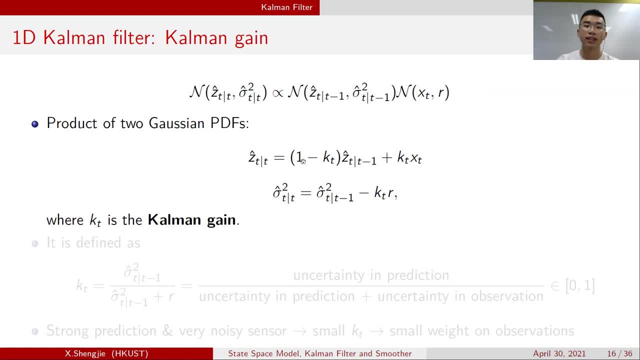 and their weight is controlled by KT, And KT is in fact a common gain, a really important concept in common filter. And as for the variance and variance, it has this relationship. So 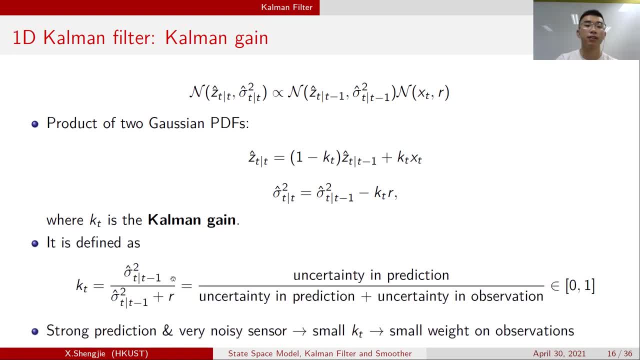 how does this common gain define? Common gain is defined as the uncertainty in the prediction We have. we have noticed that this one is called uncertainty in the prediction Because it's T conditions on T minus one. 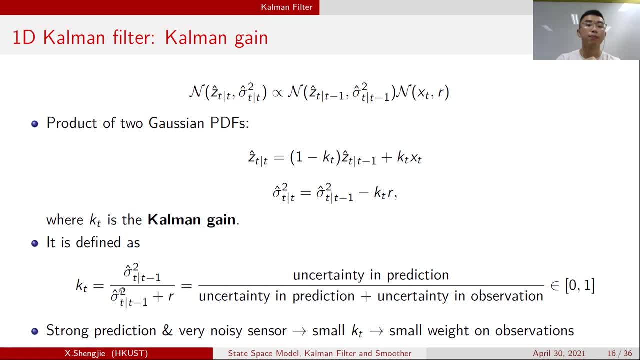 it is doing prediction. This is uncertainty in prediction And this is the uncertainty in both the prediction and the observation. So the uncertainty in prediction is a very important ratio. It relates between zero and one. 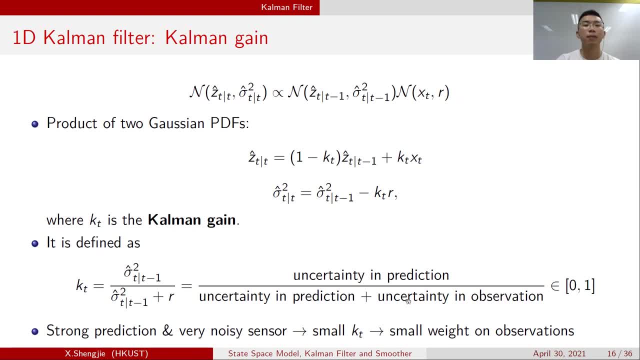 This. what's the meanings of this common gain? As you can see, the common gain means how it gives us the information of how much we should trust in the prediction Or how much we should trust in the observation. 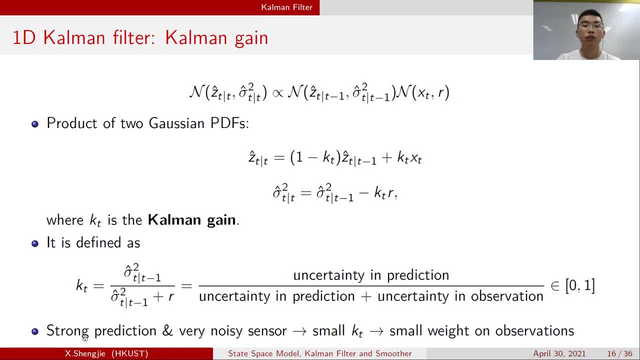 A simple example: when we have a really strong prediction, which means the uncertainty in the prediction is pretty small- And a very noisy sensor- The uncertainty in observation is pretty large- Then this common gain will become pretty small. 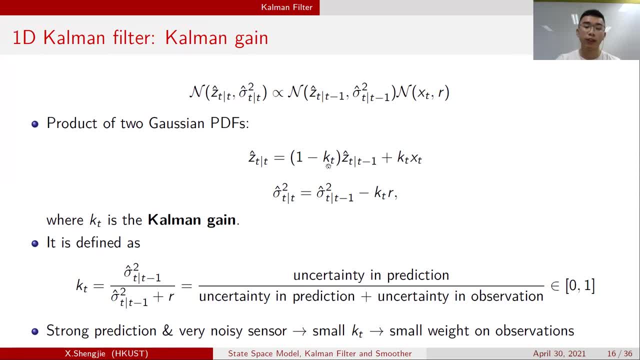 As when we and we look back, if the common gain is pretty small, our correction will mainly lays on the prediction, But not but forget about the observation. So you can see the the effect. 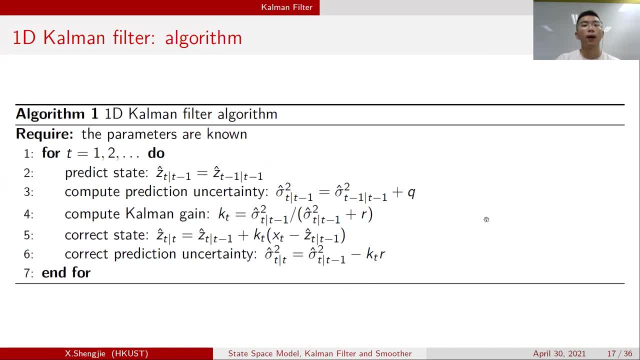 It's like a switch, And so when we sum up these algorithms, prediction, correction, and it's it's quite simple, Just a few lines. In the line two and and three, they are doing a prediction. 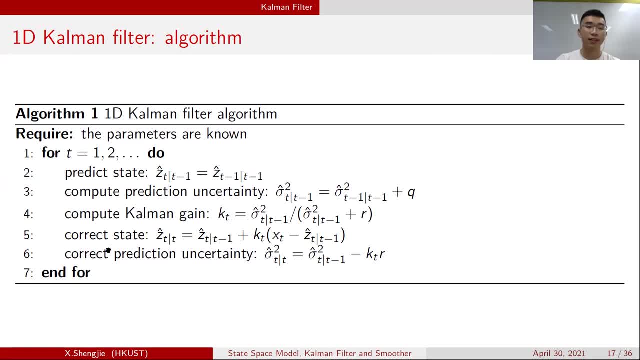 Predict states, predict uncertainty, and four, five, six are for correction. We first we have to come compute how much we should trust in the prediction, Or how much we trust in the observation, And then 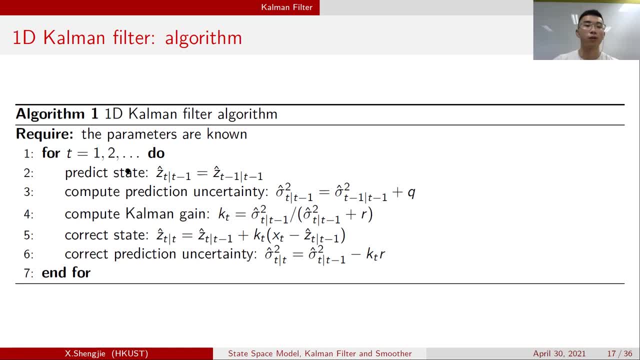 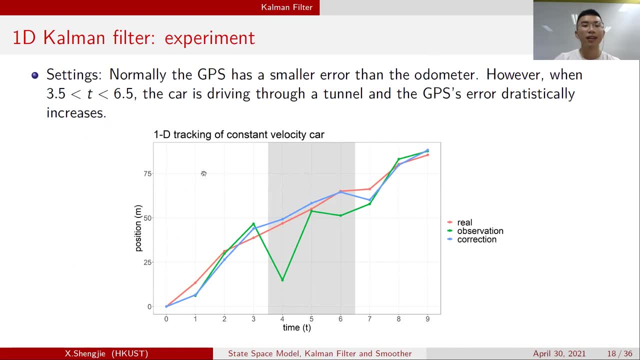 we will do the correction, We would correct the state and correct the uncertainty, And then this is the intuitions of the common future. Let's have a look at this experiment, Consider that, consider it is. 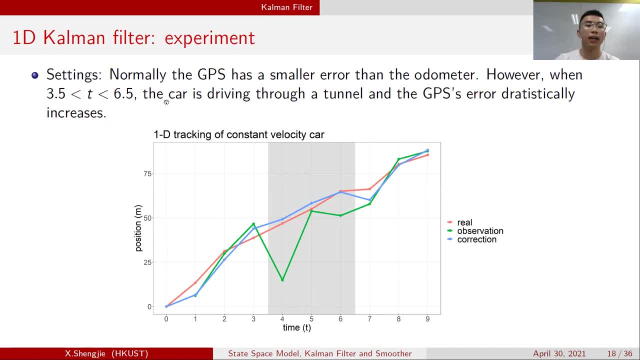 it's the the same as the previous previous example, But now we have some settings. Consider that GPS. our observation has a smaller error than the of the odometer in the in the state equation. 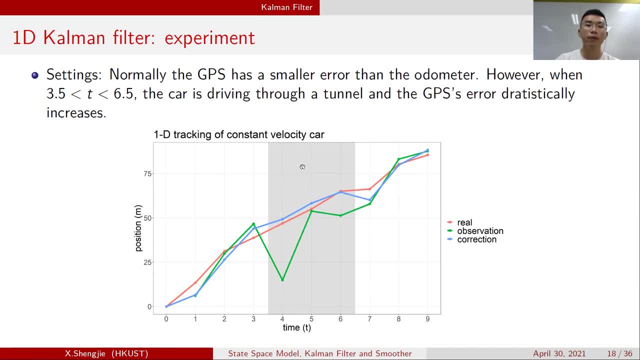 GPS is more reliable. However, during the gray area, the car is driving through a tunnel And so the the GPS error drastically increased. So, as you can see from the plot at the beginning, I 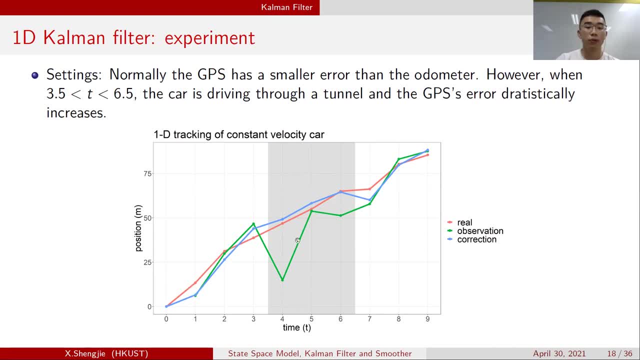 I should clarify first. The red one is the real. is the real state or the real location of the car which is hidden from us? We cannot see it. It is just generate. it's a synthetic data. 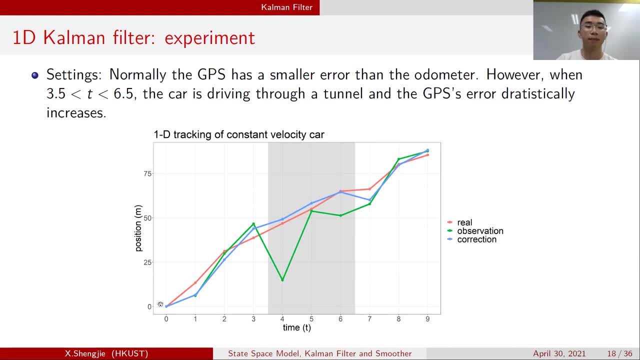 but we don't really know. in fact, We cannot see it And what we can only see is: the green line is from the GPS, is the observation from the GPS And, as you can see, when we trust, 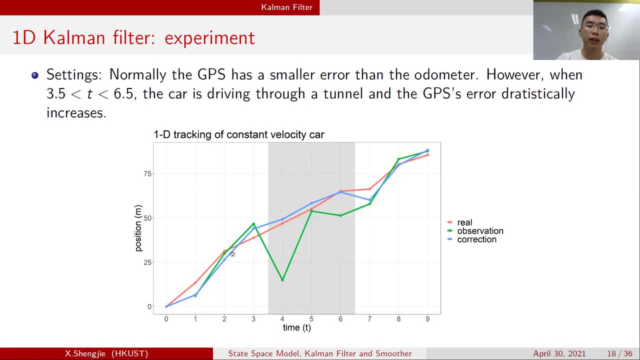 at first we're pretty trusting the GPS. So our green, our blue line. the result of the common filter is almost the same: It follow the trains of the GPS. But when the car drive in the tunnel, 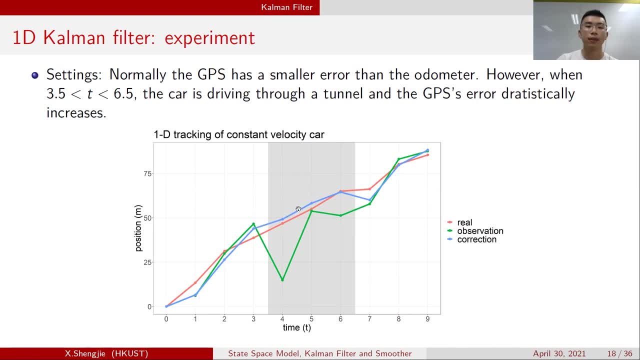 we will forget about the GPS, We will follow the state transition, We will follow our prediction. We will not believe in observation anymore, And so the common filter would go this way, this way, this way, But when it? 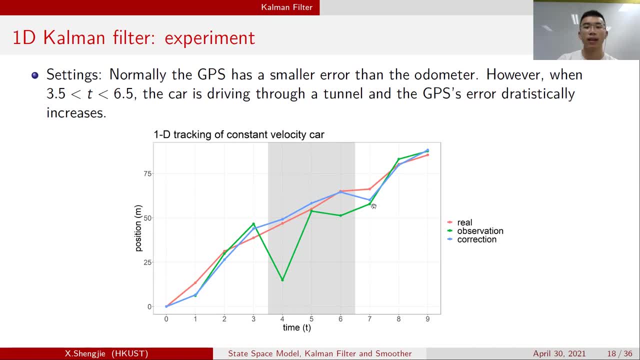 when it go out of the tunnel. we will again, we will try to believe in the GPS. So, as you can see the result of the green, of the blue line, the common filter has a really great 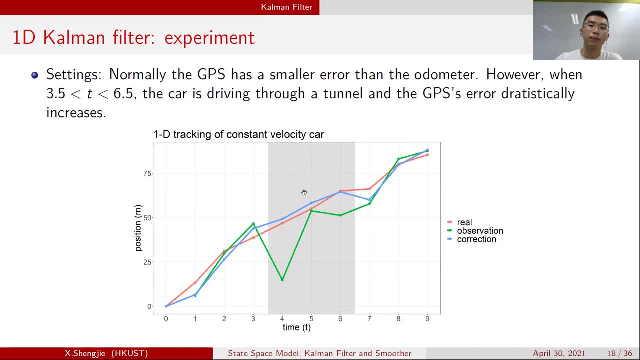 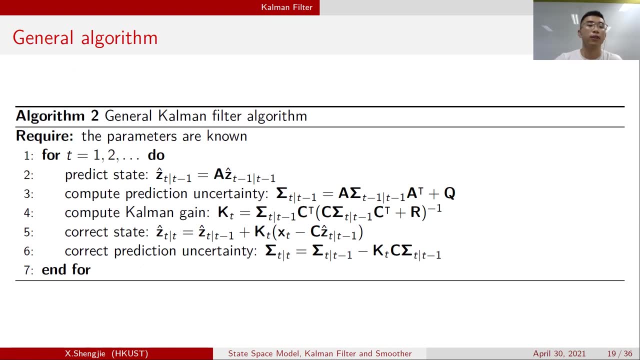 approximations of the real position. So this is the powers of common filter A more general algorithms. the general state-based model is: all is almost the same: Two, three, four for prediction five. 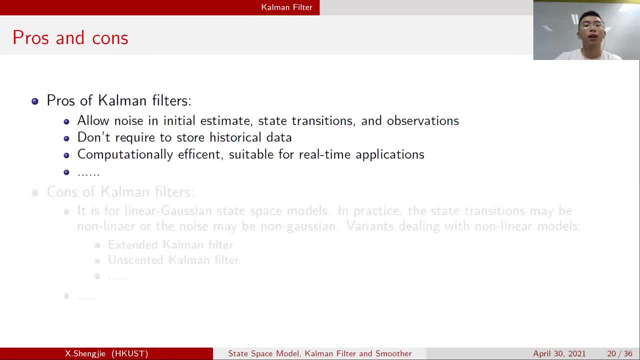 four, six for correction. Yeah, You don't have to get into the details, And so, in summary, what is the pros and cons of the common filter? The advantage is that the common filter based on state-based model. 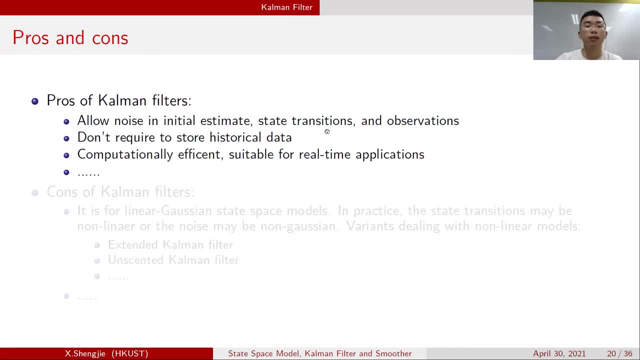 And the state-based model allow noise in initial estimate, in state transition and also observations. So it's a really well-designed model and you can use in many cases. Okay, And common filter is the optimal. 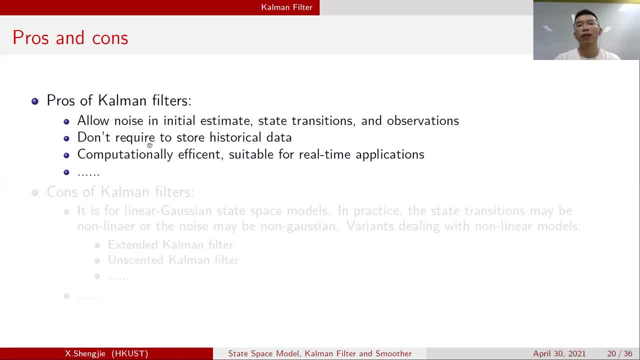 solutions of this model. And the second advantage is that it doesn't require to store any historical data, Because when we do a forward, when we, when we doing the forward loop, a forward flow, we only need to update. 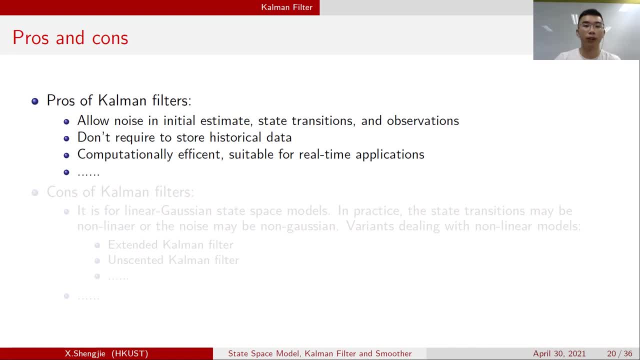 our previous state and then predict and then update, predict. We don't have to store our previous states because of the marker property In the hidden state. So the third advantage is that it is 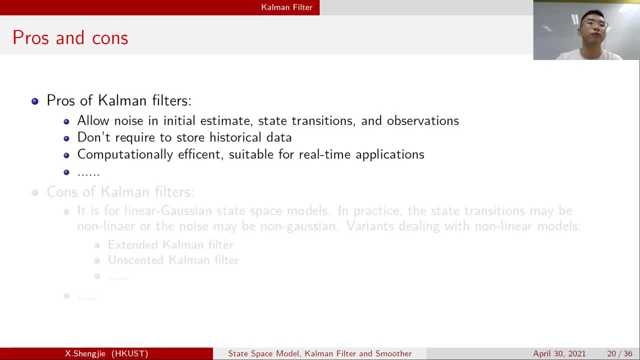 computationally efficient. It's pretty fast. Just fill lines and forgot about the previous data. So it's it's widely used in a real-time application, For example, our self-driving car- nowadays pretty popular And 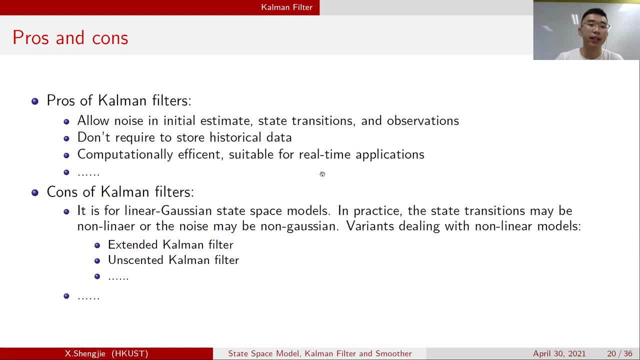 the cons of the common filter, or we call it the limitations of the common filter, is that it is designed for linear Gaussian, state-based model, But in practice the noise may not be Gaussian And the state transition. 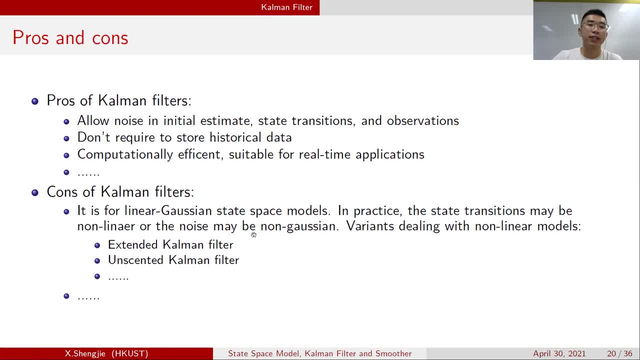 may not be linear, So use the traditional common filter is limited. Well, people have developed some variants to cope with this kind of problems, For example the extended common filter, the unscented one and particle filters. 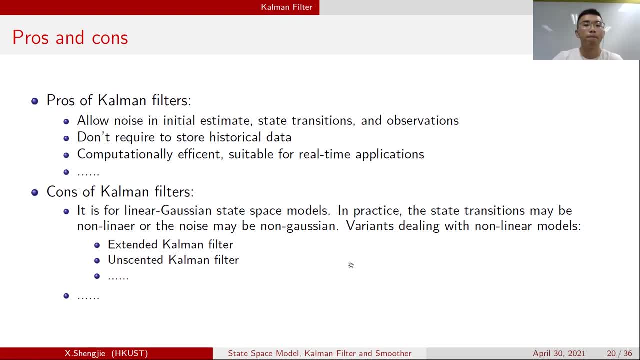 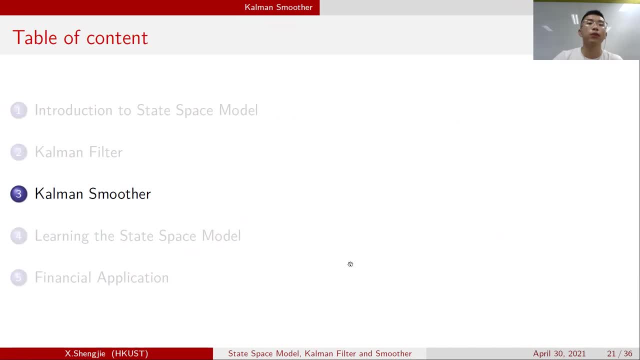 And it's also a good choice. So this is all about common filter. In the third part we will go into the common smoother Before we get into the details, And actually I really not talk about the detail. 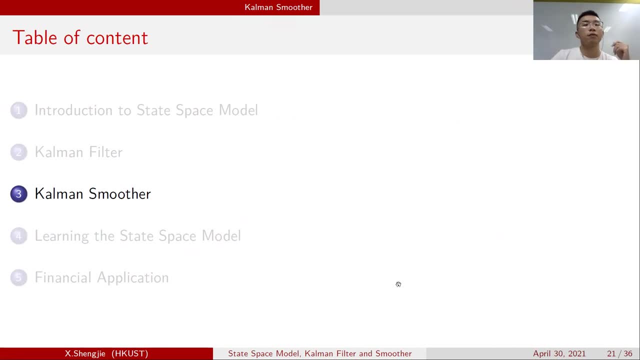 because it's quite complicated. We should refresh our concept: What is smoother? What is smoother is to trying to get a better estimations of the state previously, After we have. we have this observation. 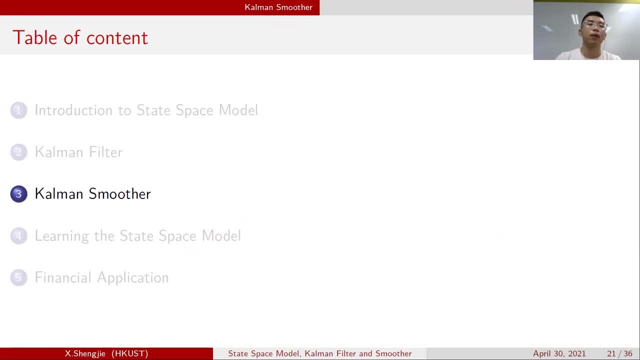 So what is when we should apply it? Consider if you're in a, in a, in a hedge fund or in. you want historical data of the previous year, the whole year, And you want to. 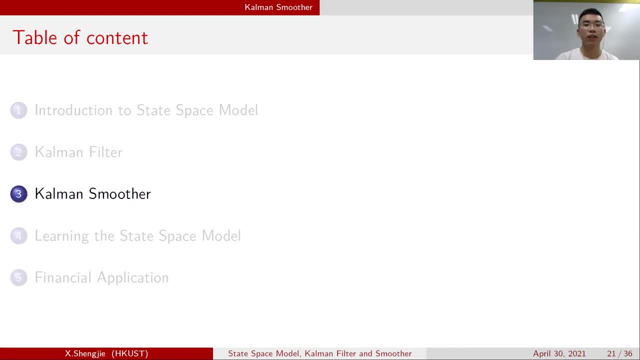 find out the hidden information in the previous year. And so, in this case is you are doing analysis. You are not doing prediction, You are, you try to analysis, analysis that the performance of the previous year. 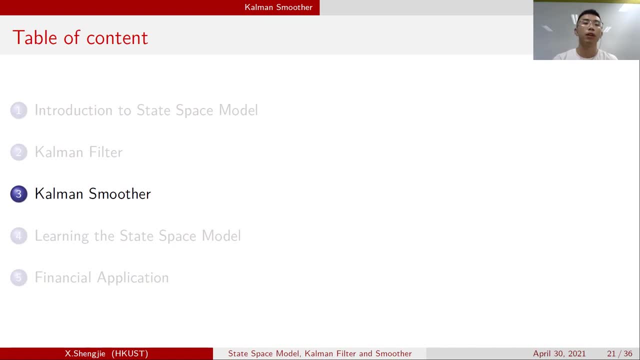 And then- this is the case when common smoother comes in- It will try to but help you to find out all the hidden information previously based on the whole year data. So here here I will give you the 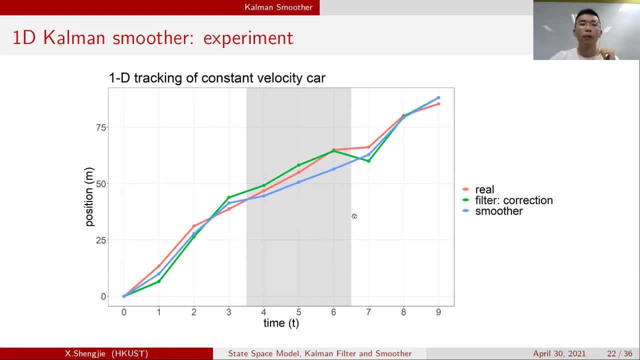 the. the same example as before, the car driving through a tunnel, But right now I will show you the the performance of the smoother. The red one is still the real position. The green one is the common filter. 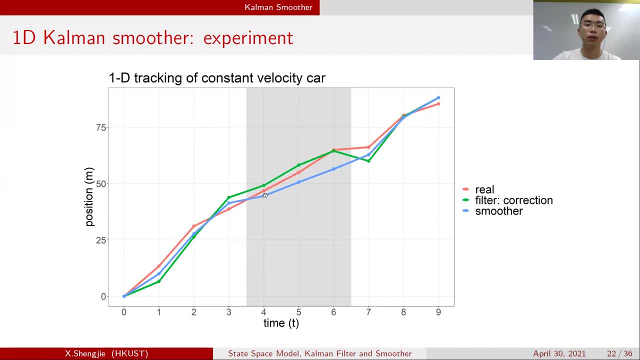 And the blue one is the common smoother. As you can see from this case, the common, the common smoother will will provide, will provide much smoother performance than the filter And for example, here: 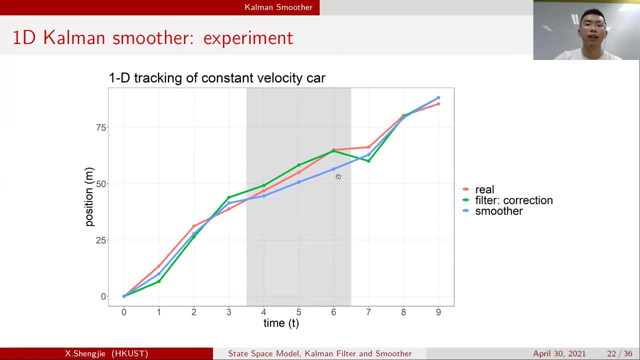 the filter suffer from downward trend, which is not what we like, But in the in, the smoother- we have already solved this problem. It becomes smooth- and provide a better approximation And so, generally speaking, the. 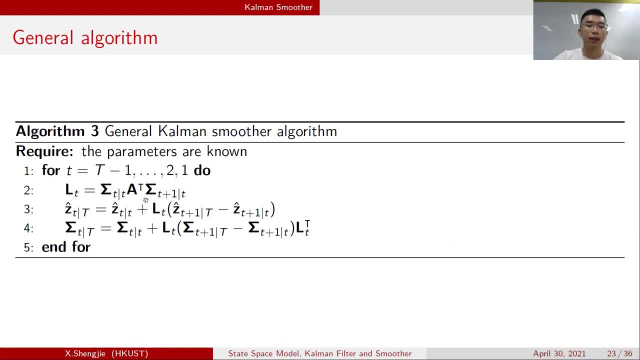 the common smoother can be written like written like this, And it's a a backward flow algorithm. But before we we run the common smoother, we have to do the forward first. So common filter is always be. 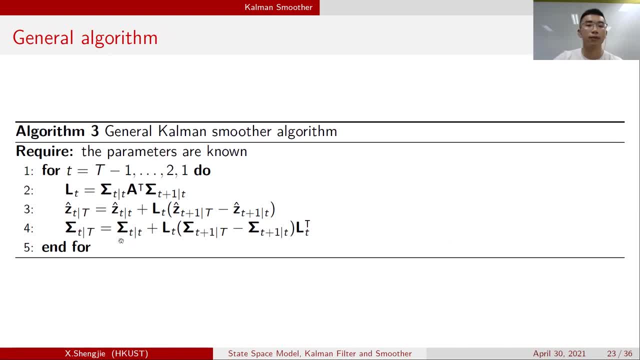 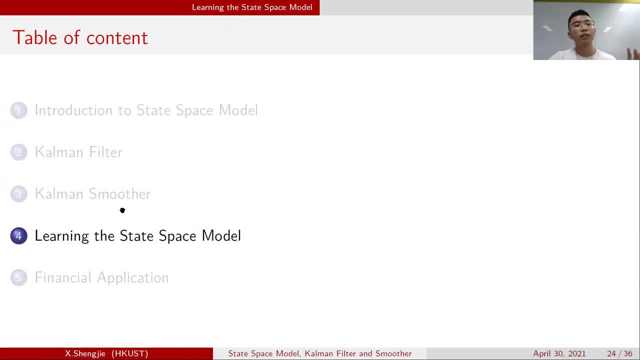 before the common smoother. You don't have to get into the details of this, this equation. And in the fourth topic, in the previous case, the common filter and smoother. we assume that we have already know the parameters. What is parameter? 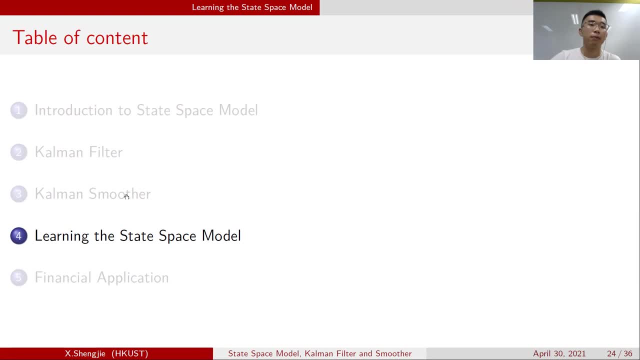 Parameters is just when you are, when you are doing a portfolio design, portfolio optimization. You already know the parameters- mu parameters, sigma- But in practice, you, you, you don't know, you may not know. 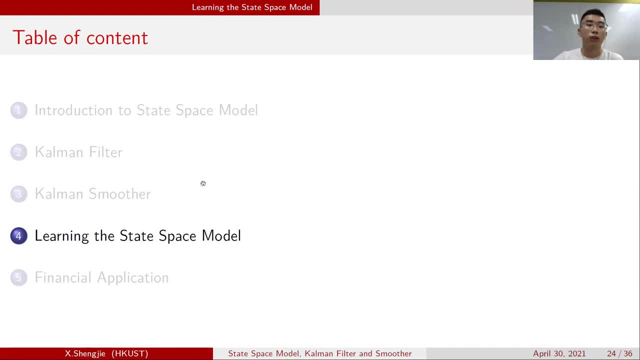 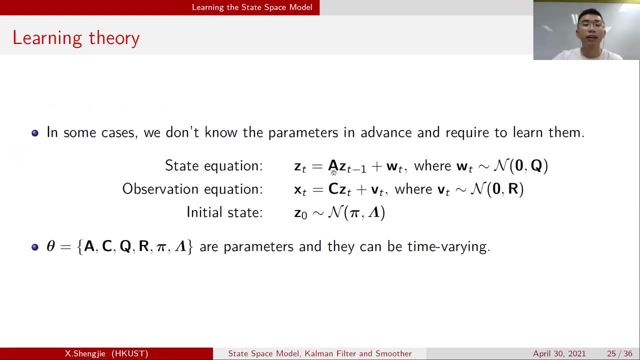 you have to use some tricks to train them, to find them, And this is called learning And we have to learn. for example, in this state-based model, there are some parameters. The A is the parameters, the transition. 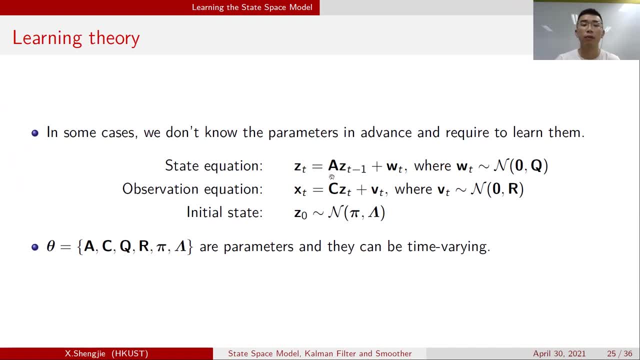 But in reality we don't know the transition How. but although we, in our first example, we know that, okay, the transition A will be one, But in fact we don't know in some cases. 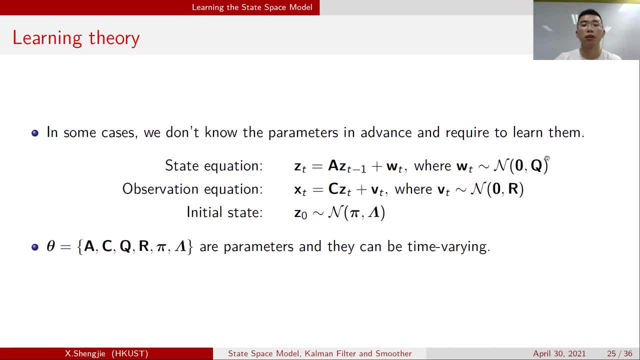 in most cases, And we we may not know the noise, the, the co-variance of the noise. we may not know that, So we require to study these parameters from our training data to help us to build. 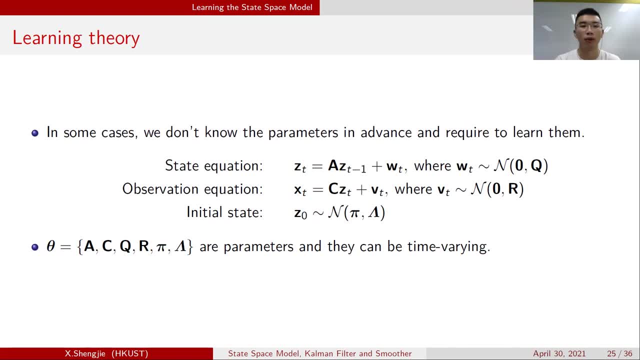 a, a complete state-based model, And these parameters can also be time-bearing, And so the the problem is how we try to learn them, how we learn them When we start off our, our learning theory. 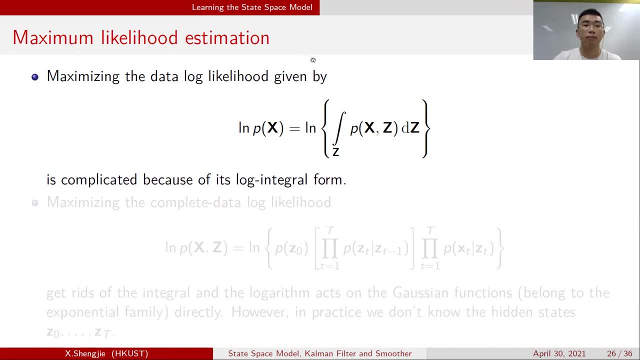 the most important one is called the maximum likelihood estimation, Which means we're trying to maximize the data log likelihood. It's written. it is written written in a, in the following form: And as, as we can see, 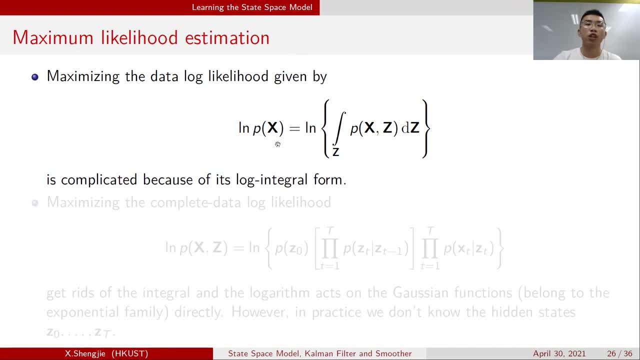 our, our objective is: is the data log likelihood, the data likelihood And in most, in practice, we don't know the probability of the data. We only know the probability of the, of the join of the. 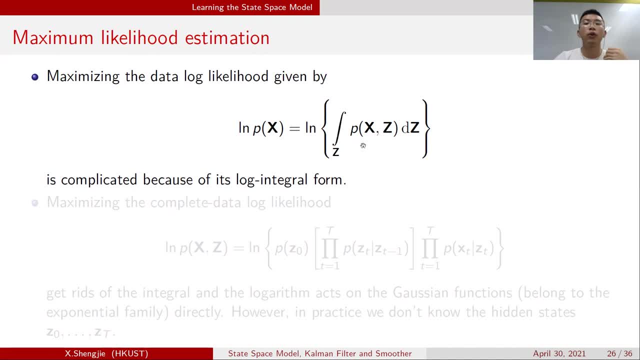 hidden state and the observations. So we have to take the integral to get this Px. Forget about the log. So we have to take the integral to get this Px. So we have to take the integral. 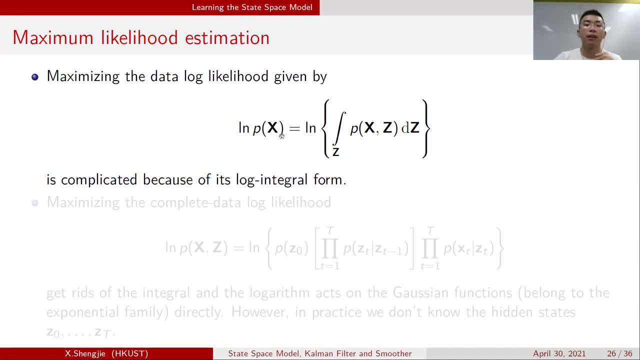 to get this Px. Forget about the log. Yeah, And the problem is that this integral is pretty difficult to calculate, So this may not be a good choice. We may not directly maximize this data log likelihood. 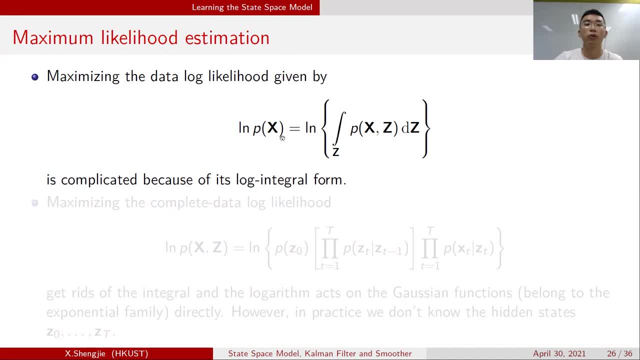 to find out our parameters. So, alternatively, if we know the hidden states, we can try to directly maximize Px state, the joint probability, Because this has a really elegant form. So if we know the hidden states, 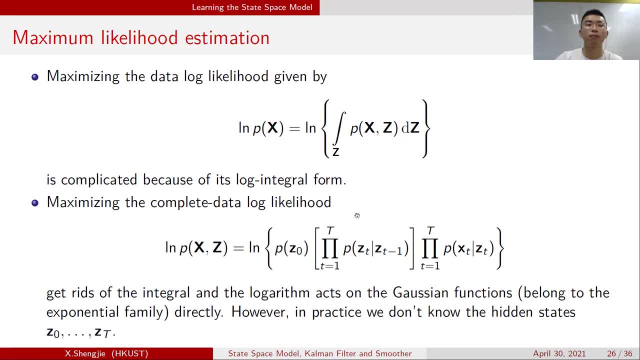 we can use a really elegant form, as you can see here. Well, the problem is that, in practice, we don't know the hidden states, So how we can find out the parameters. This is when 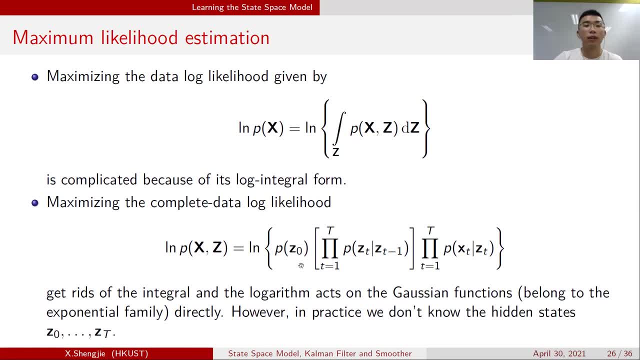 the expectation maximization algorithm comes In this case. we don't know the Z, But we can calculate the expect value of the Z. We may guess a Z. So this EM algorithm is doing. 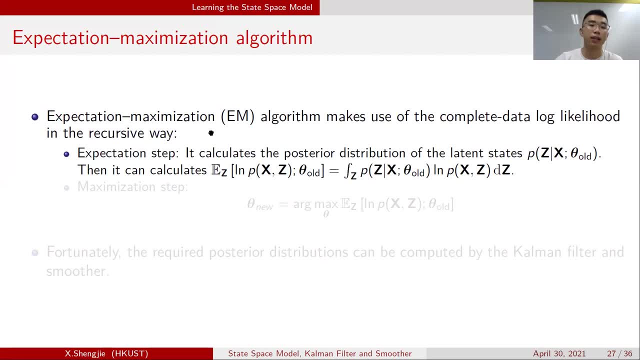 this, like this EM algorithm- expectation maximization, Expectation step- if it has two steps- One step is expectation step- It will calculate the posterior distributions of the latent state Denoted as P. 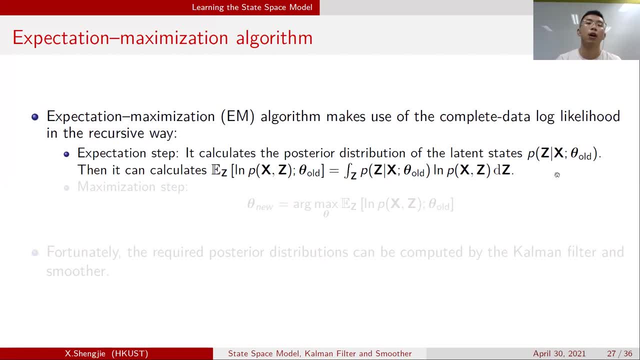 Z, conditions on X. So what's the meaning? It means that we have these observations, we can predict the state. Well, we have a guess of the Z And then, by the guess, the Z. 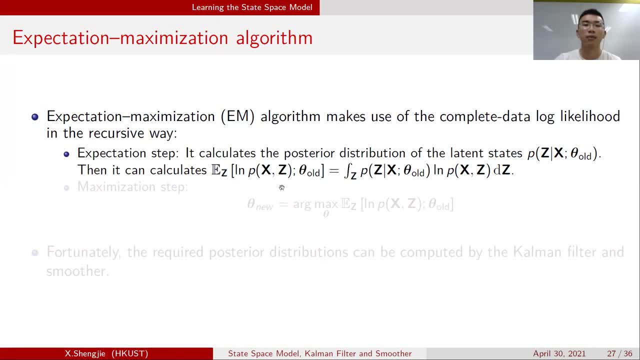 we can calculate this log likelihood, The objective of our, our MLE, And in the M step it's just directly maximize this expectation. In most cases, this maximization step is pretty simple. 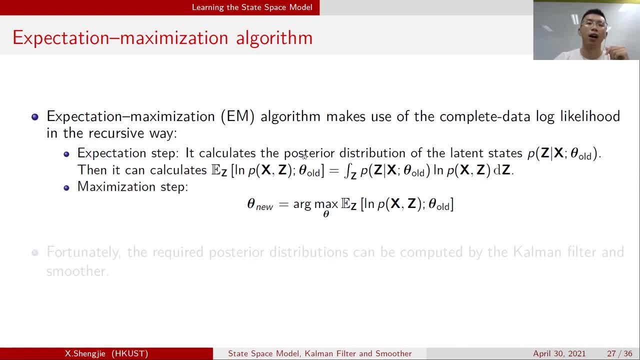 It always has a close form solutions. But the problem is that how we can find out the posterior distribution, How we can guess the state from all the observations. In fact we have already done that With the common filter. 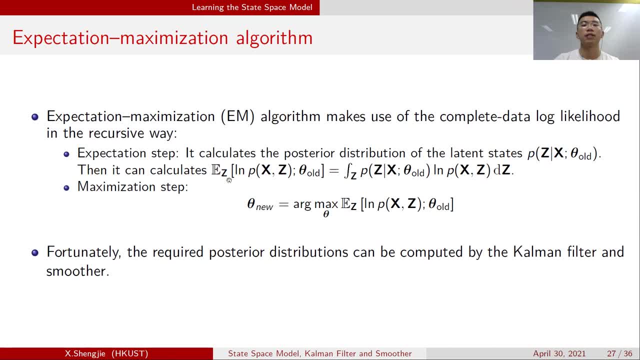 and common, smoother we can calculate the, the expect value of the states, Because, as previous chapters we have talked about, talk much about how we can guess the state from our observations. This is, this is: 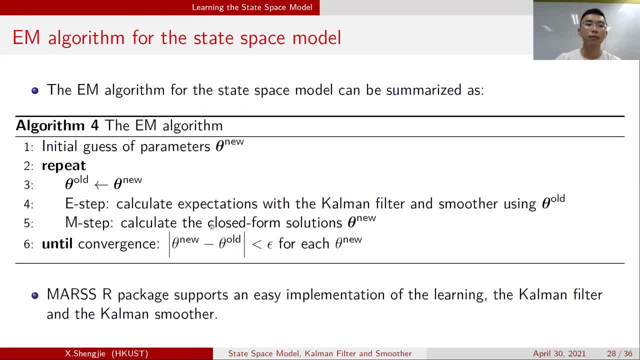 when it comes in in the learning theory. So the EM algorithm can be summarized as the following: We first have an initial guess of the parameters, Then in the E-step we use the common filter and spoofer. 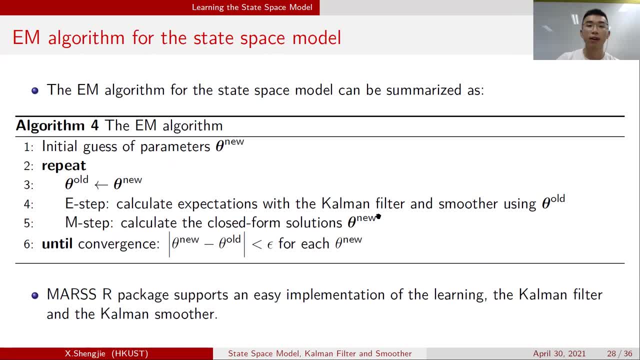 to calculate this, to inspect their probability, their posterior probability, And then we can calculate the expectation of the complete data log, likelihood, our objective function, And then in the M-step we will optimize it And 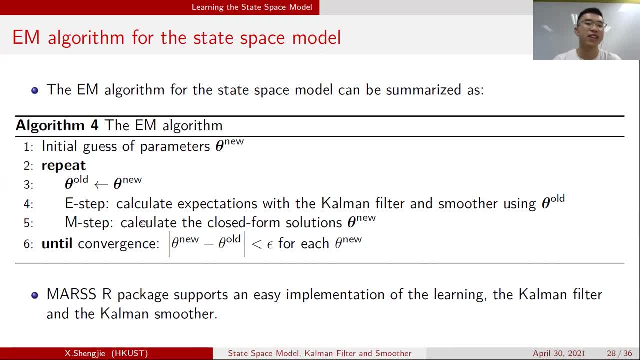 we don't have to use CVX to do that, Because it has a closed form solution And we can simply write it out. So it's pretty simple And these new estimate parameters will feedback. 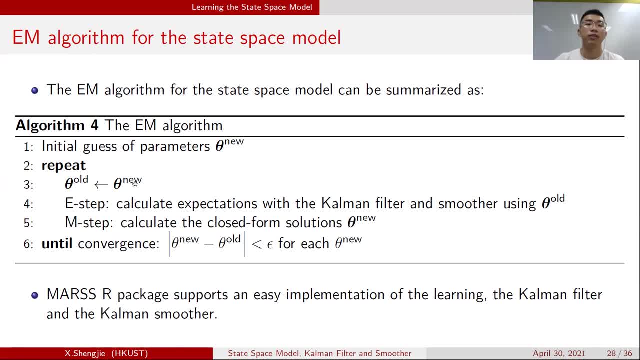 Because, you know, the initial guess of the parameters may be pretty worse. And we have we have to loop to find out whether there are better, better estimation of the parameters And finally, all the parameters. 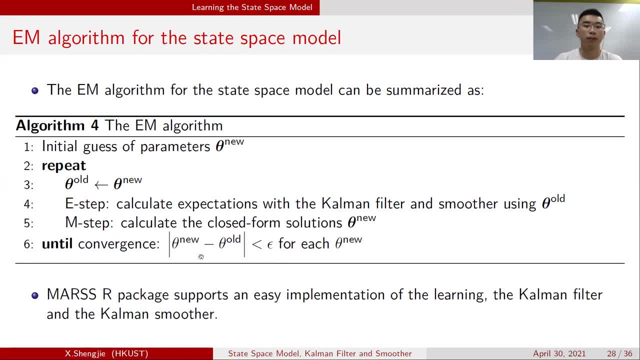 will converge. So this is the ideas of EM algorithm And till now we have already learned common filter, common spoofer and how we learn the parameters. All these have already been coded or packed. 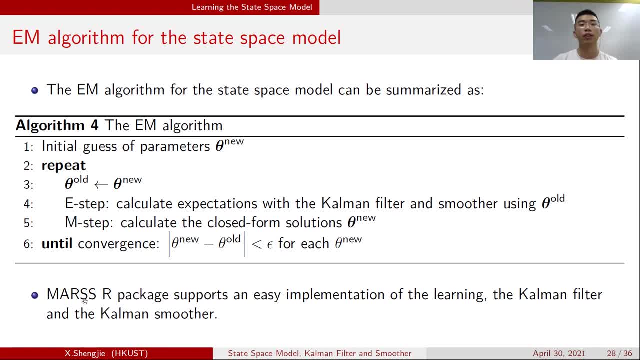 in a package, For example the R in R, there is a package called maps And it has. it can support a really really easy implementation. It has a. it has a clean interface. If, if you want to use this, 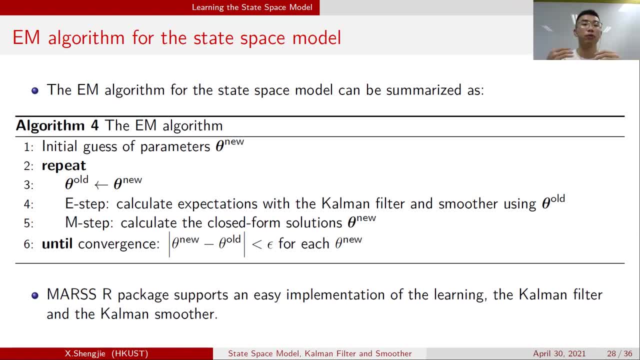 state-based model. you can just simply define it And they will train it for you And they will move it for you, And you don't have to worry about your your coding. So it's pretty easy to. 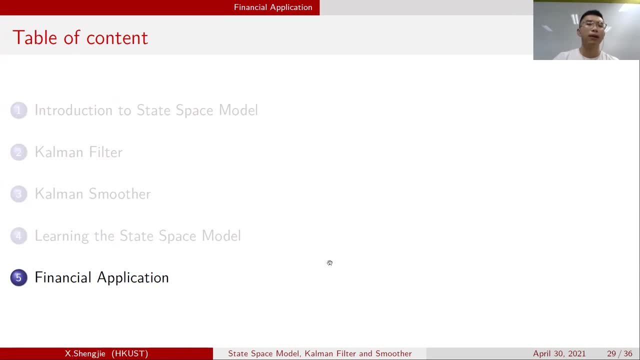 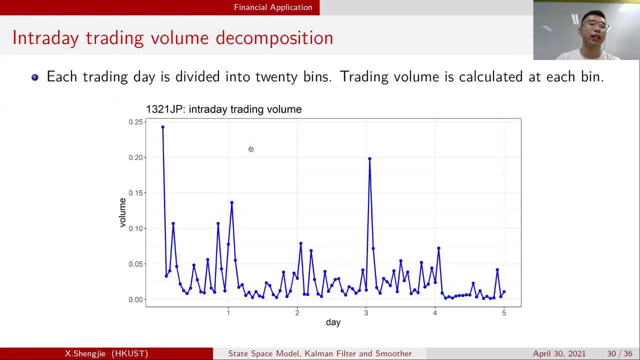 implement And finally, we will talk about it, how it- how this state-based model applies in finance. The one application I want to share today is the intraday trading volume decomposition. Trading volume is. 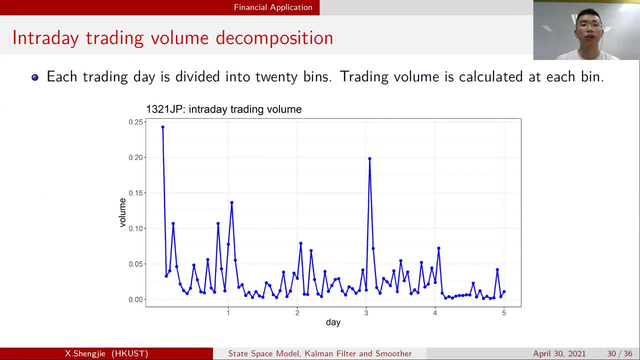 as all, I think most of you have already noted, And trading volume is showing how active your market is, And intraday here means within each day. we, we don't, we don't only have 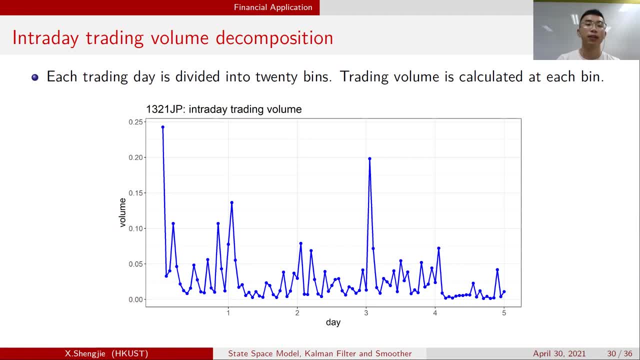 not only have one trading volume, We have sampled it Every 15 minutes we have a record of the trading volume, And so, as you can see here, this is one day, this is the second day, And 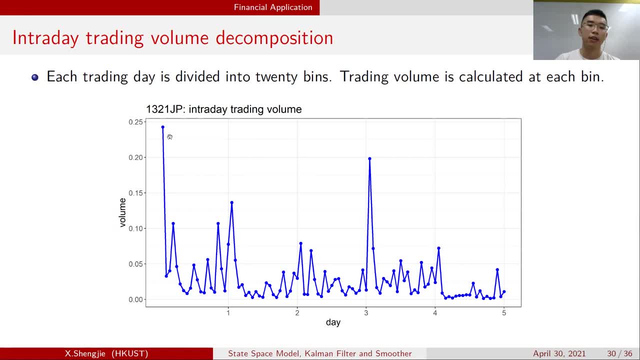 the trading volume is look like. oh it goes, because at the beginnings of the of of our trading hours the trading volume is pretty high And then it will drop down And later at the end. 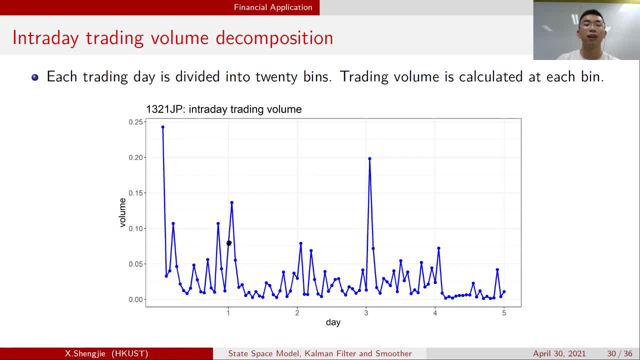 of the trading hours, it might achieve a, a peak Which is in line with our integration, And this is called a smiley smiley patterns or U-shaped pattern, And we want to decompose it. 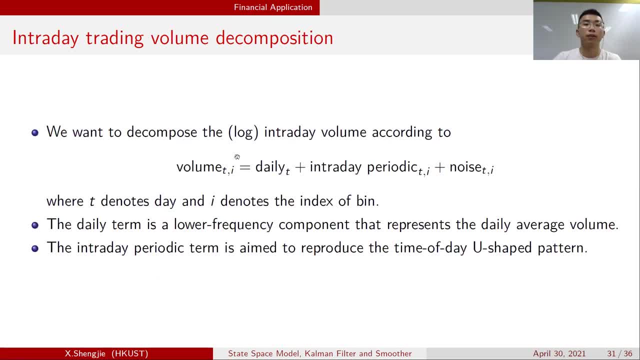 We want to decompose it in several components: Volume decomposing in a in an additive, in a in a in a an additive. The first one is is the daily component. Daily component, which is a lower. 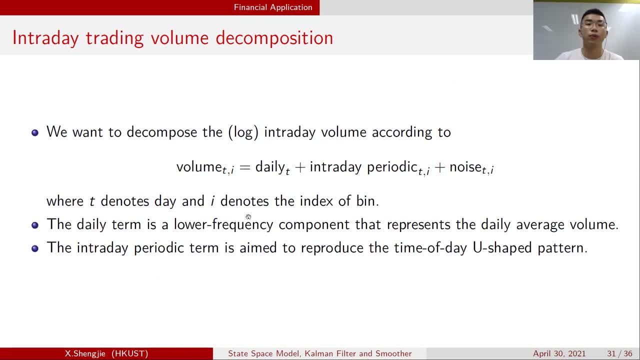 lower frequency component, which represent the daily average of the volume. Each day we have a daily component And the next day we have a max daily component. So t here denotes day And within day. 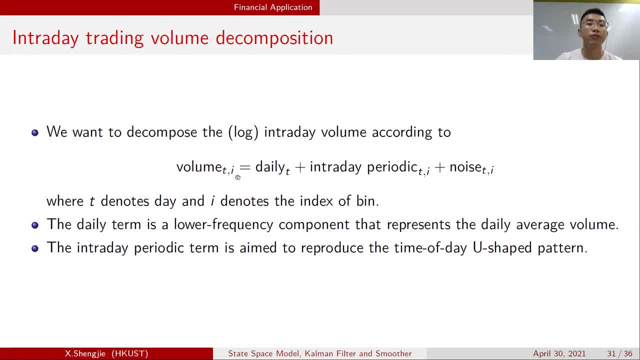 we have many bins, We have many samples And i will range from one to maybe 20.. There are 20 sample each day And denotes the index of the bin. So daily doesn't care about what's the index of the bin. 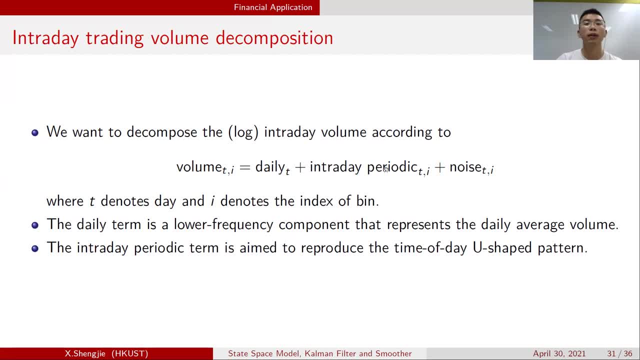 All the bins have the same daily component, But for the periodic component it cares about the bin Because when you're in different times in a day then the periodic term may be different. So this is M to reproduce the time of day pattern. 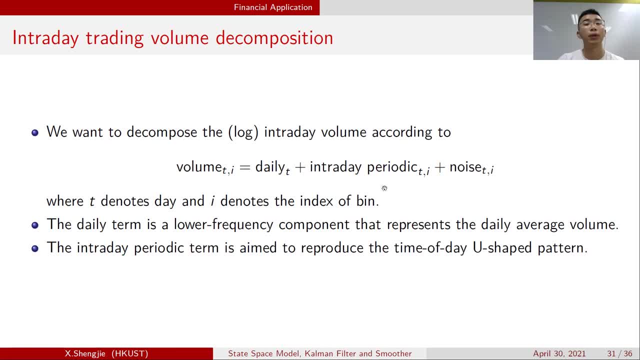 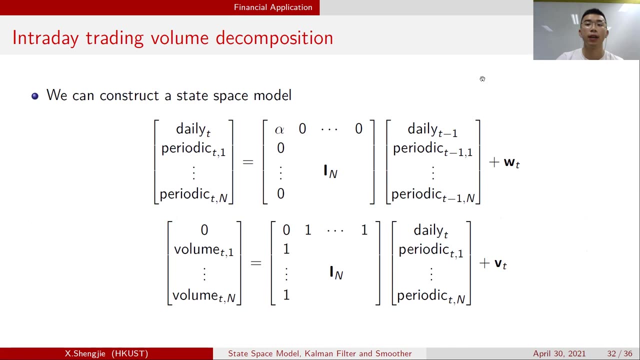 the smiley pattern, the U-shaped pattern. This is coded in the periodic term. There is another deuce term- And so we can construct a state-based model based on this assumption. For example here: this is one realization, And each moment in the state model denotes one day. 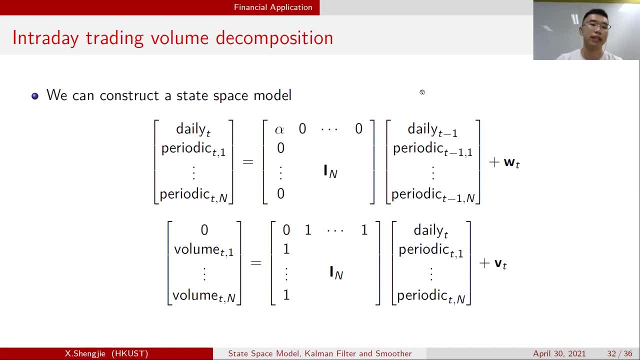 This is one day, this is the second day, One day transit to the second day And in each day there are many hidden states And the first one is the daily hidden state. Each day has a one daily term And they have N, and here denotes the numbers of bins. 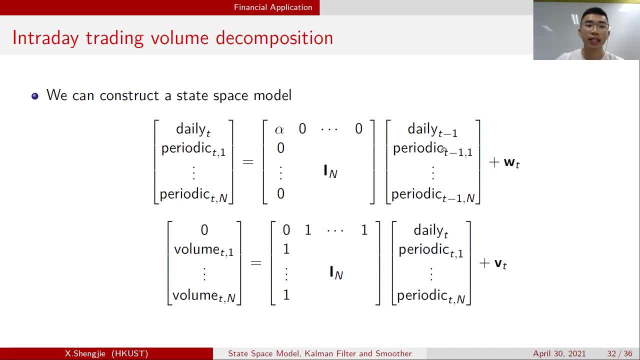 They have N periodic terms or periodic states. So here will be N plus one hidden state, And you will transit to another day How we do it. Alpha is a parameter. we want to learn. We want to find out whether the daily components will change. 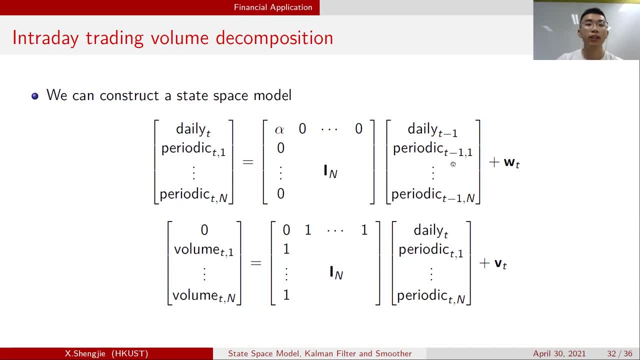 ways that they work. Is that their ratio? but in, but for the periodic term, which is you can see here, is that identity matrix, each periodic term or each bin. we hope that it looked the same because it is one. We want it to stay the same. 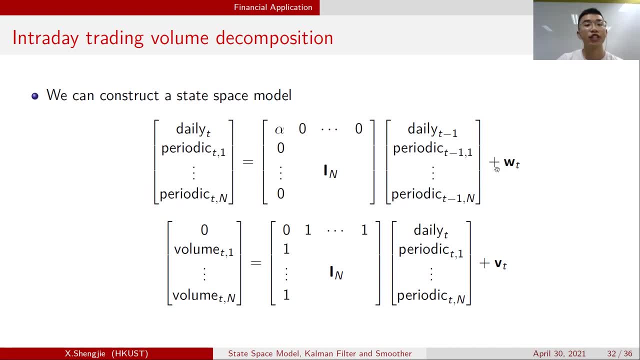 but here we allow some noise and definitely it can change a little bit, but not a huge change. So this is the meanings of these state equation And for the observation it means each volume. each volume is a combinations of daily and a periodic term because, as we can see here from the 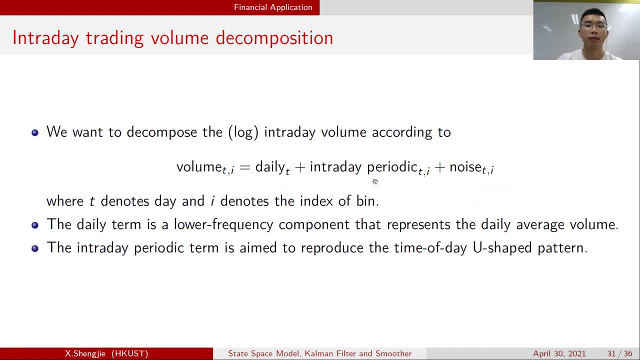 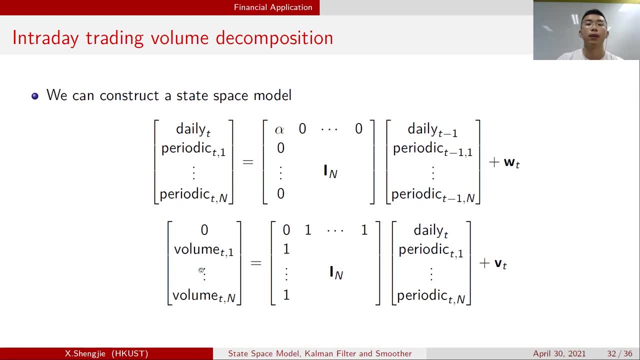 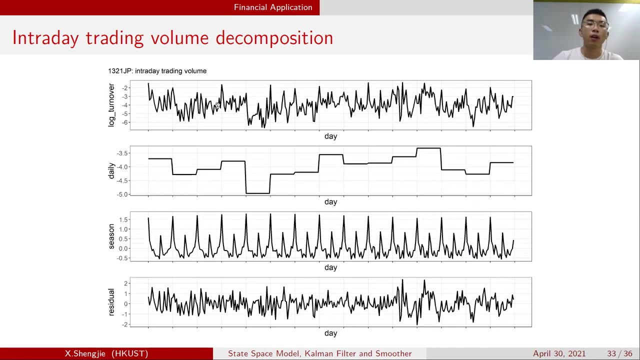 from the addictive model: daily plus the periodic. So here each volume is the daily plus one periodic. This is a diagonal matrix and this is the way we can drive state based model. How it perform. You can see the result for the log volume. 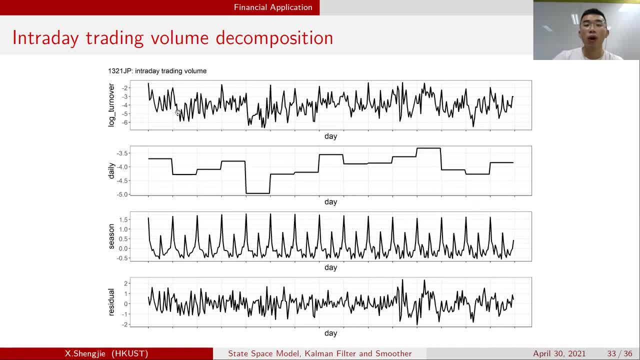 The volume we put here now. this is the log volume. after running the common filter and smoother, we can get the decomposed result: the daily term, the seasonal term and the residual term, which we think is the noise In the daily term. 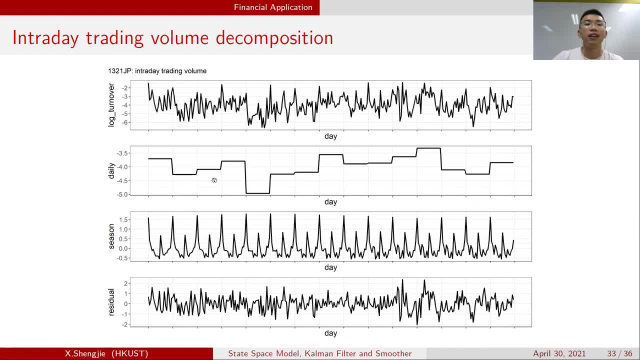 you can see it is like stairs and it is what we want. It depicts the daily average of the volume And season. you can see the seasonal term. it looks like the smile face or W shape- U shape doesn't matter- And we can find out this hidden information from looking in depth. 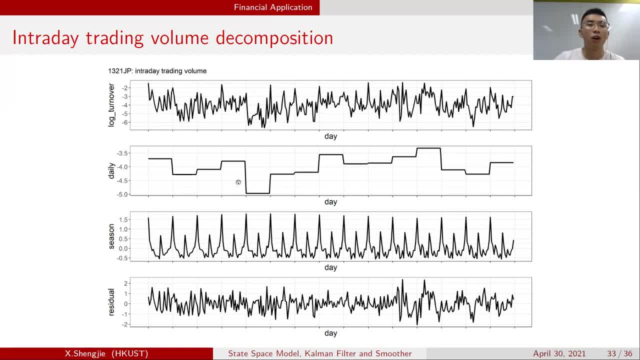 In this really, really noisy signal we can extract two really important hidden information by constructing a space model And in the residual, the noise. we hoped it to look like a white noise And yeah, it's pretty noisy and nothing. not many valuable information can be. 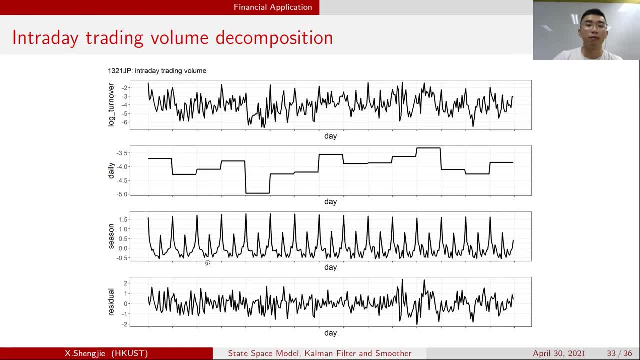 found here. So this is the powers of common filter and smoother, So okay. one thing, Although we want to, this is designed for decomposition, but, as we can see, we can do a time series forecasting. How do we do forecasting in this example? 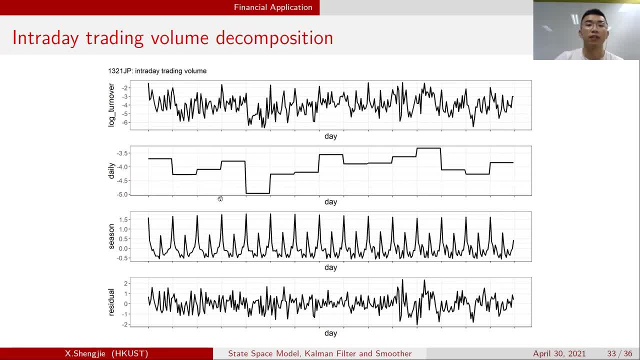 I believe that we have already, in our homework, we have done something similar. We try to decompose a signal and then we like to predict. predict the trains of each component. For example, this one is when we fit an AIMA model on it. 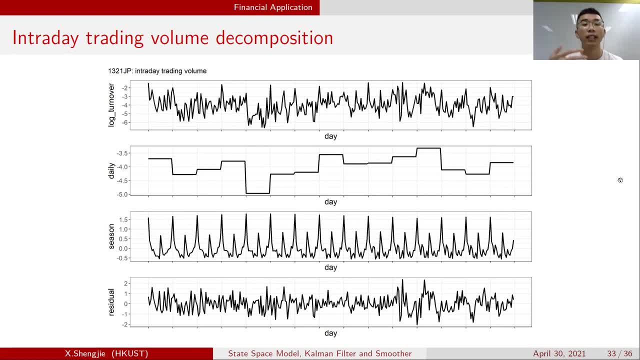 it would look like this, So we can predict the future daily term, how it looks like in the future, And the seasonal term. we can keep it the same: This amount of phase, this amount of phase, this amount of phase, So the predictions of the future trading volume. 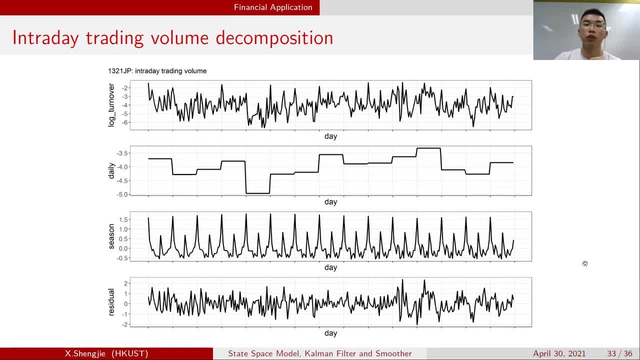 can by simply add up these two terms together and set the noise to be zero, And results have already shown that using this method outperform all of the other methods in trading volume prediction. So this is the power of state-based model. So, and I think this is the all of today's tutorial, 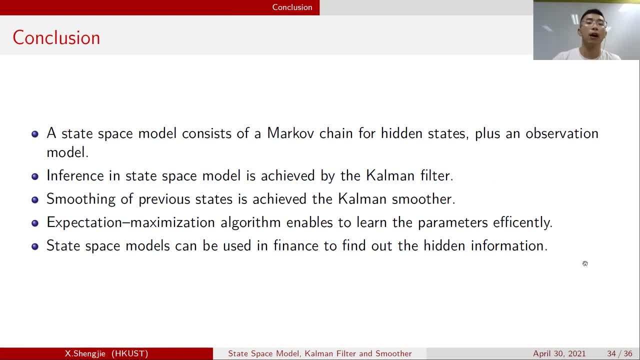 and I will give you a conclusion. The first is that we talked about the state-based model. It consists of a marker chain or marker, a hidden state that follow marker properties and then plus observation model, which is how we observe from the state. 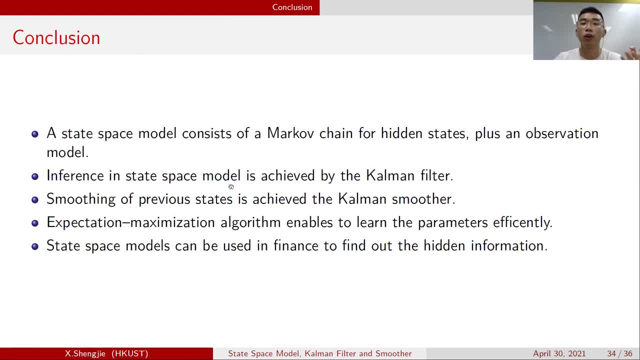 And inference in the state-based model or the forward algorithm is called a common filter And the backward one. so the smoothing one is called the common smoother And the EM algorithm help us to learn the parameters efficiently And the state-based model from our application. 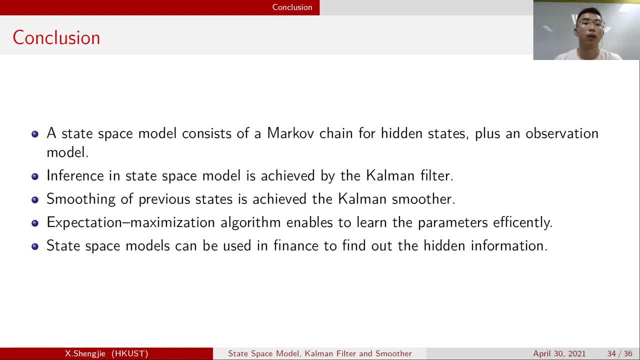 you can see that it's quite useful in finding out the hidden information. So when you want to use this state-based models in other financial application, it's pretty simple. You can construct a state-based model, or perhaps you don't know which state you want. 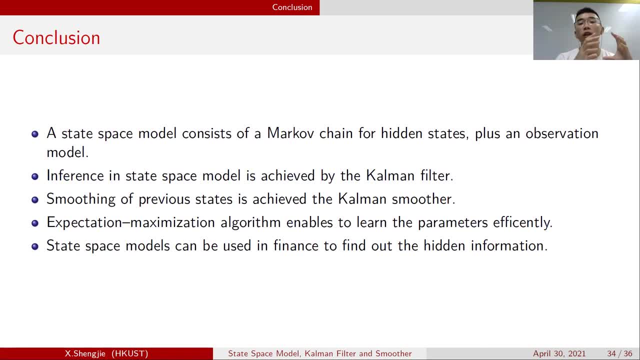 You can just put, you can have a try. put some states. You may not know how the transition of the states from T minus one to T, how to change it. You can set it as a parameter and you can learn it with EM algorithm. 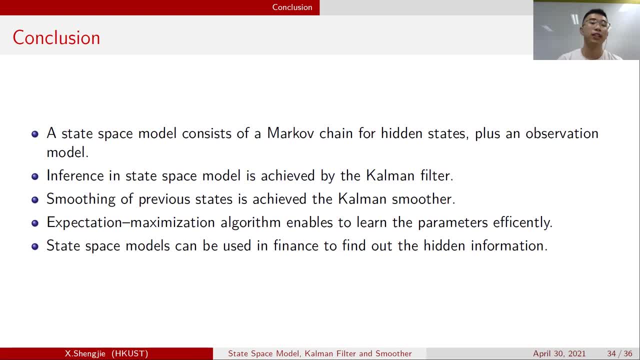 And you know, and in this way you can find out the hidden informations in some observation. For example, you observe the price and while this matter, you can find out something below the price, something more than the price, for example, whether the some trading patterns inside it. 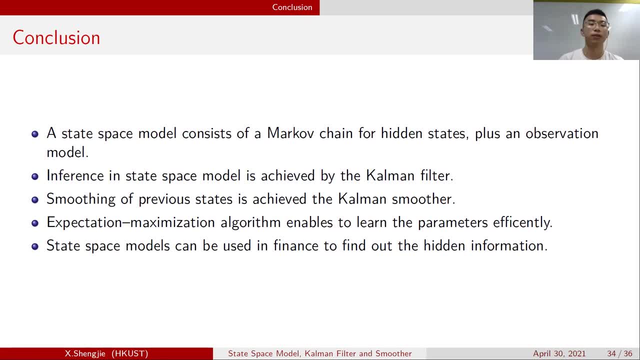 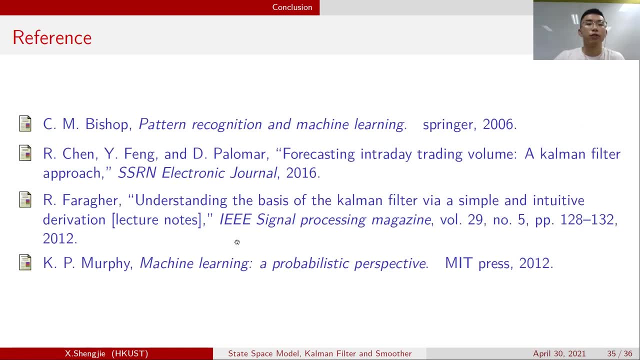 whether it is a bull market or so on. So this is the powers of state-based model And if you, if you want, if you want, you can go deeper in these links and you can find out more information in Kalman filter. 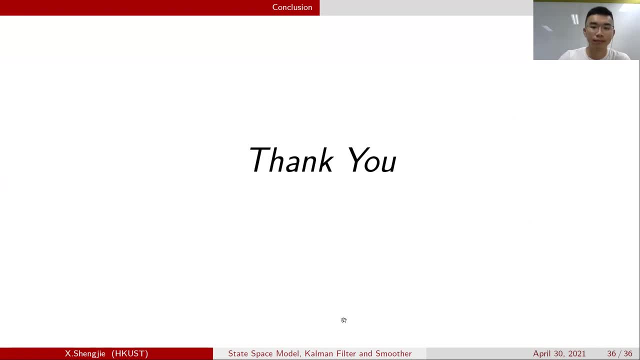 So thank you for your listening. Okay, thank you very much, Zhenzhen. Anybody has any question for him? I want to. I want to say that the Kalman filtering is really a very useful technique, very versatile, It can be applied in virtually any area. 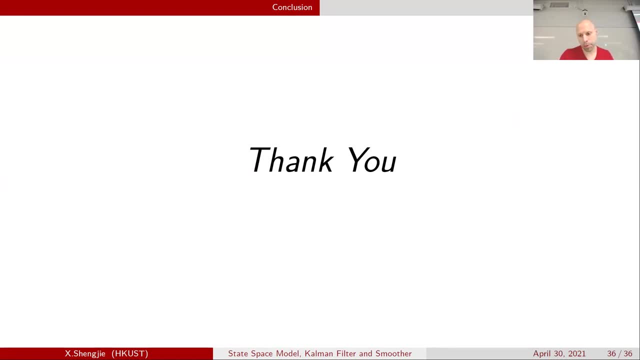 Initially it was proposed for ballistic purposes- right To control the position of missiles and planes, spaceships, many years ago in the early sixties, in the early sixties. So we are talking about, yeah, a long time ago And more than half a century ago. 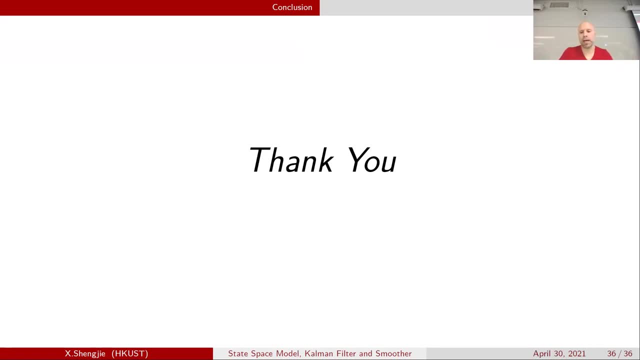 But now it's used in every area And, of course, in finance. it has many applications. So Zhenzhen has shown you just one application in finance, right for the volume modeling, but it has many other applications. Definitely it's a bit sophisticated. 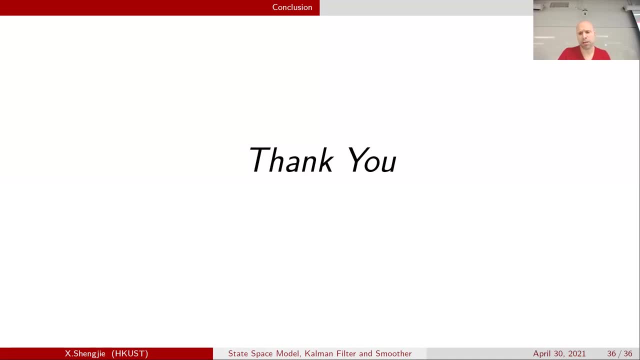 for the scope of this course. This is an undergraduate course, So it's too much for this course, but at least it's good to know that something like this exists, right, It's good for you to know. It's good to know this. 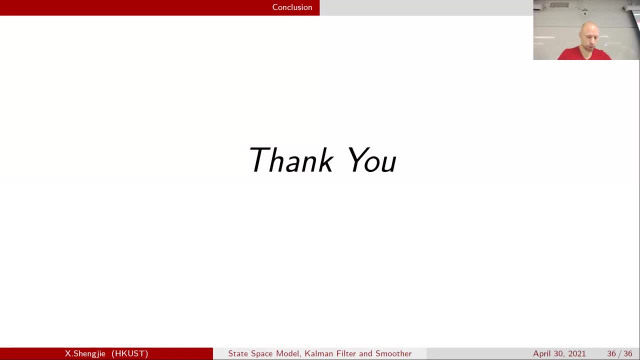 Anyway, if there are no questions, then we can stop here. Yeah, any question? Then I guess, since, like you mentioned, this method was developed in like the 1960s, then has there been like newer methods have been developed. Zhenzhen, you wanna reply to that? 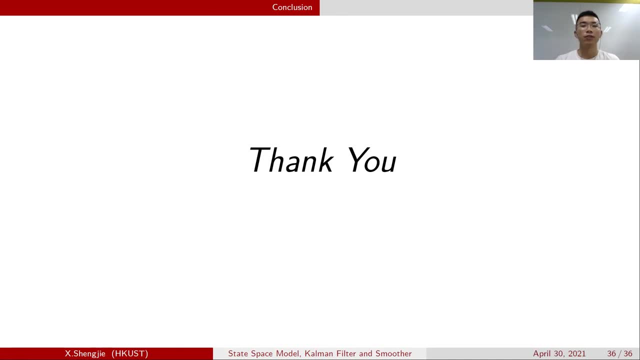 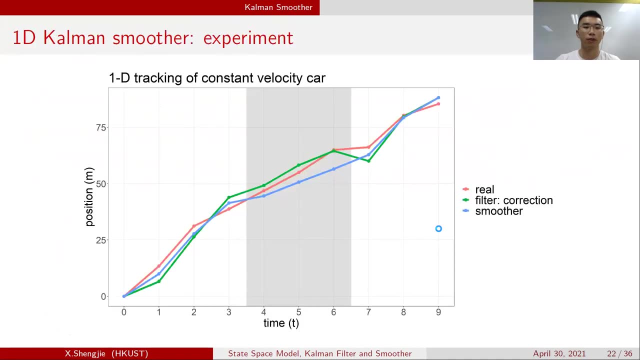 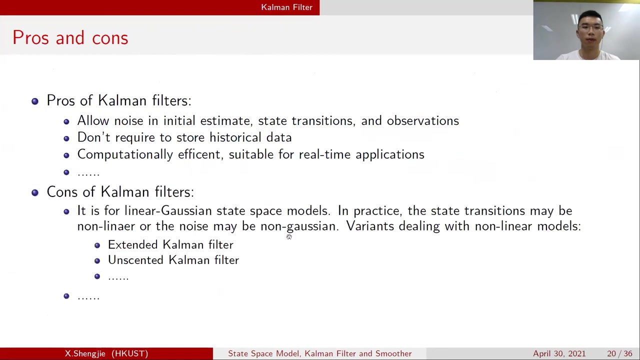 You wanna reply to this? Yeah, yeah, In fact, a common filter. we have shown that before. there are some variants to deal with different kinds of problems, as we have, I'm sorry. Yeah, And the common filter is designed for the easier case. 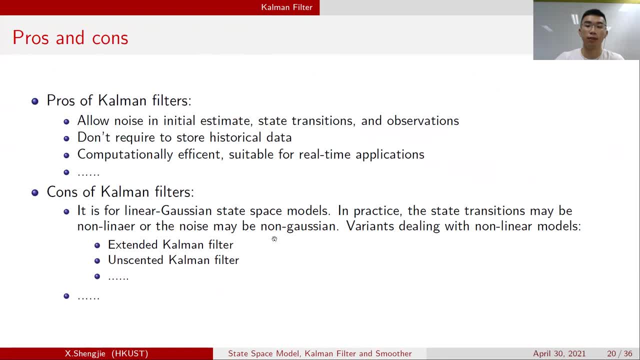 And in practice, your models may be more complicated, And so you can use some other variants of the common filter we have shown here. And I know that you mentioned the common filter is designed in 1960, but definitely there will be something new. 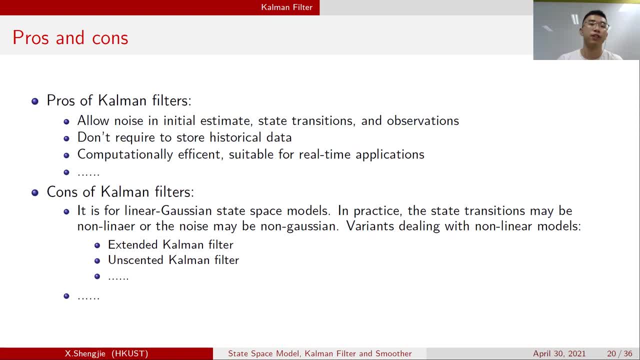 but it is nothing about common filter, because common filter is one optimal solutions of the state-based model. So you mentioned that there may be some model that replace state-based model. This is possible And there are some. there are definitely some other models. 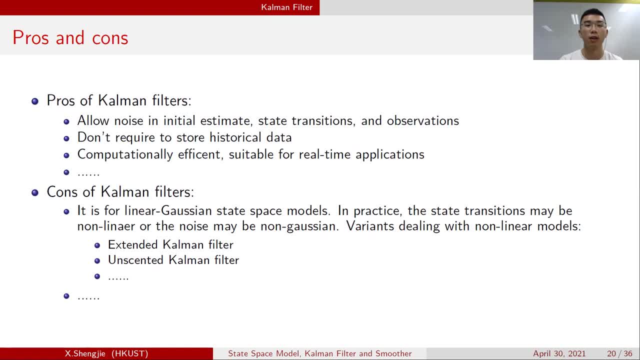 to try to model the word in different ways, but for the common filter itself. common filter is the optimal solutions of the state-based model. So you can find a better solutions of the state-based model, Yeah, in a literature. So let me repeat just to clarify what you have just said.